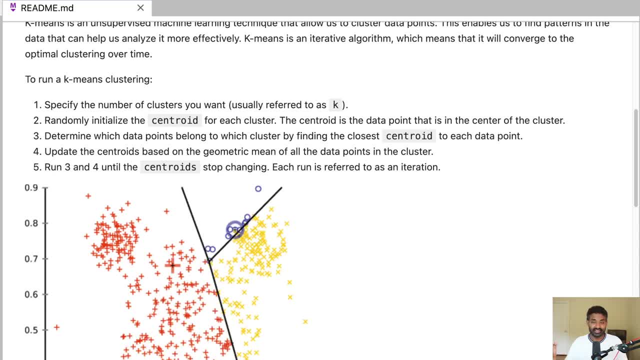 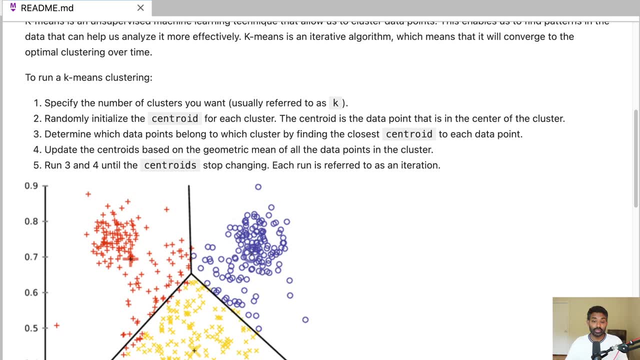 number of clusters you want, which is what k means. So k can be 3. if you want 3 clusters, 5, etc. Then what we do is we randomly initialize the centroid for each cluster, And the centroid is just the central point in each cluster. If we look at this gif, the centroid is represented by the black. 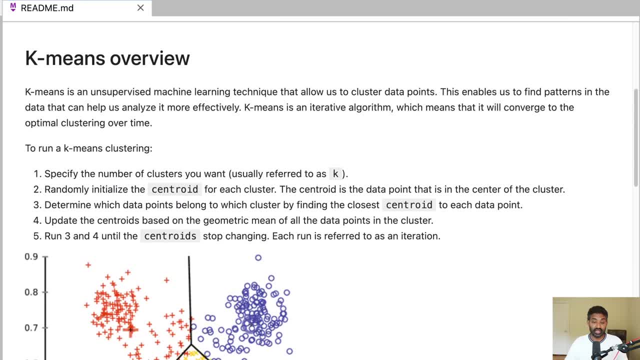 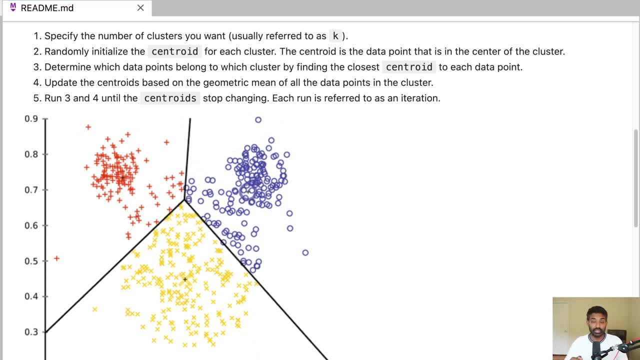 plus sign And that just corresponds to the cluster center. Once we initialize the random centroids, then we determine which data points belong to each cluster. Once we do that, we can assign labels to each of our data points based on which centroid is the closest to that data point. 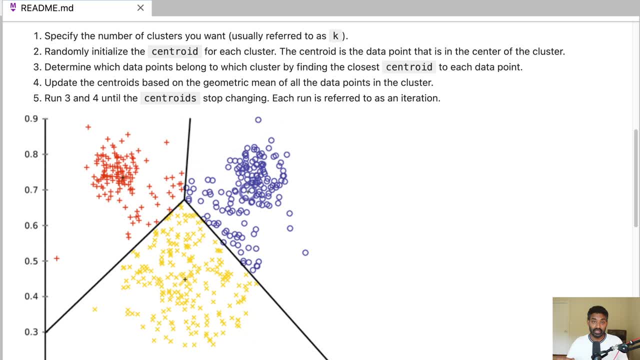 Then we update our centroid and we can assign labels to each of our data points based on which centroid is the closest to that data point. And then we run steps 3 and 4. We continually iterate until the centroid stop changing And ideally you'll hit a point where the centroid actually 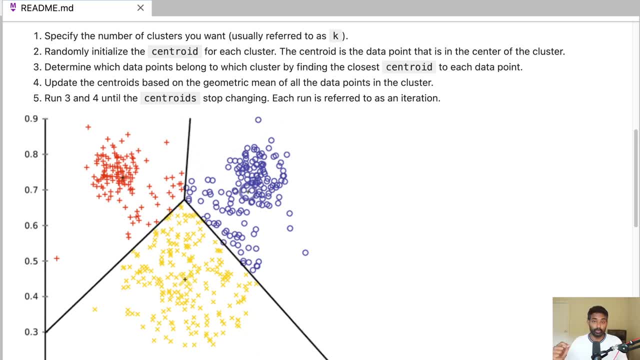 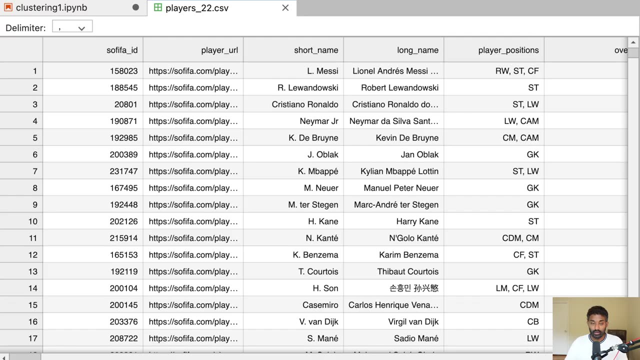 stop changing and your algorithm has converged towards stable clusters, And that's when the algorithm is complete. So we're going to implement all of this today And let's go ahead and dive in. We're going to be working with player data from FIFA, a popular football video game. 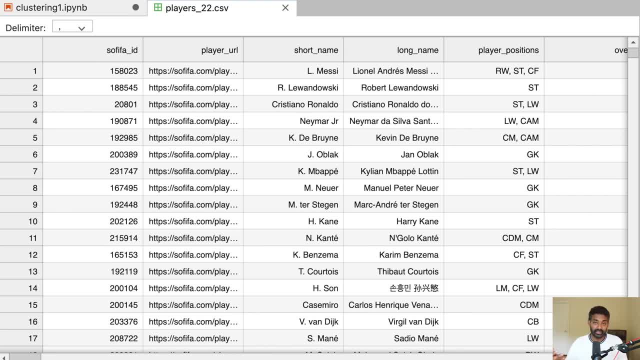 And we're going to be clustering the players And that's how we're going to test our k-means clustering algorithm. So in this data set, each row is going to be a specific player. So this first row is Lionel Messi. the second row is Robert Lewandowski. 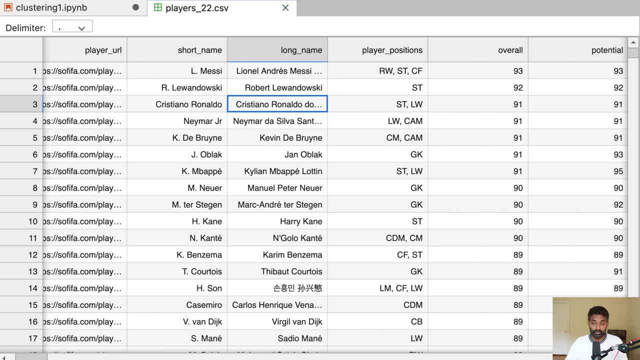 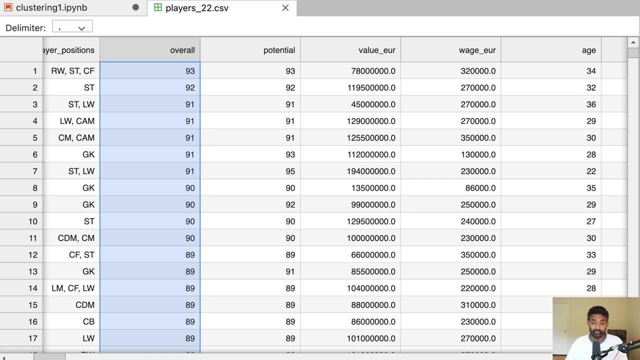 and so on, And each column corresponds to some attribute of that player: The positions they play, the overall rating in FIFA, etc. The five features that we're going to look at for clustering are overall rating, potential rating, so the highest rating they could achieve in the future. 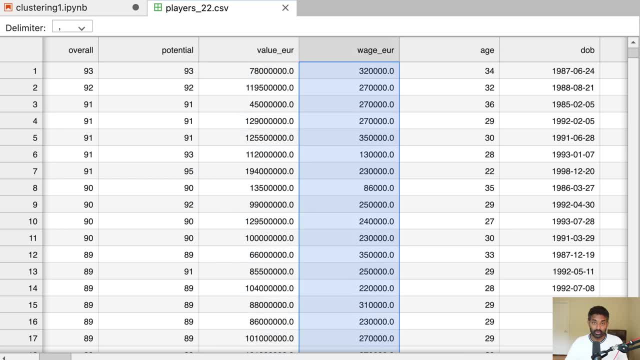 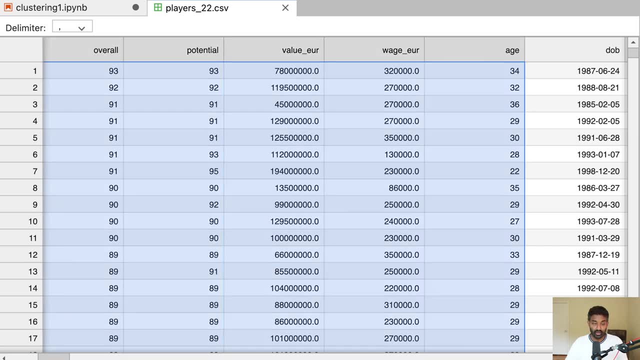 their value to their current club, their wage- so their annual salary- and their age. So we're going to cluster players based on these five features. The first thing we're going to do is just read in this player data and clean it up, And then we'll implement a k-means clustering. 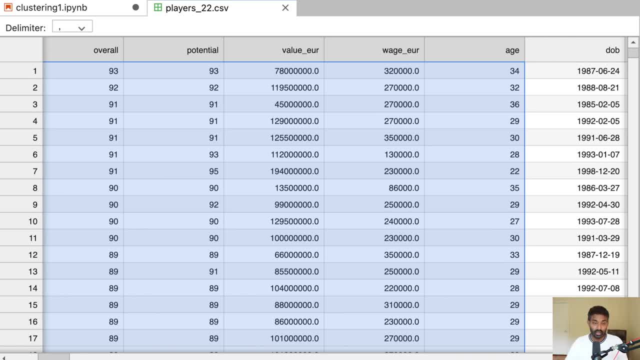 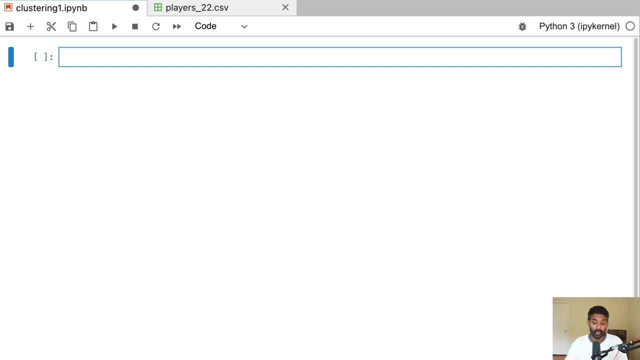 algorithm to actually cluster the players. So I'm using JupyterLab, and this is just a notebook open inside JupyterLab. You can use Google Colab, you can use Jupyter Notebook or you can use JupyterLab or any other IDE that supports Jupyter Notebooks, And the first thing we'll do is we'll import. 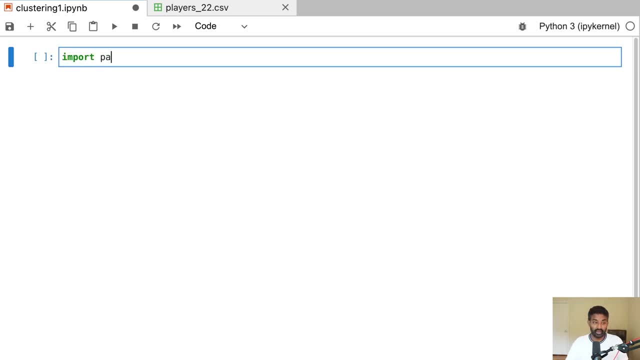 pandas and numpy. So we can just type import pandas as pd and then import numpy as np, And that will import both of them And then we want to load in our player data. So that's just pandasreadcsv- players22.csv, And that's data for FIFA players from the 2022 season. 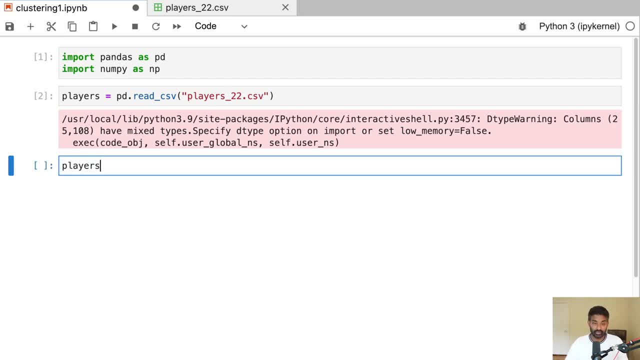 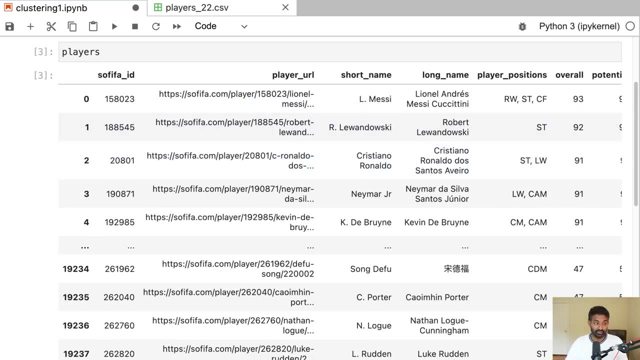 So let's go ahead and read that in. We can take a look at the players data frame and we'll just verify that it is the same data frame that we just looked at in the csv viewer. Then we're going to define a list of the features we want to cluster based on. 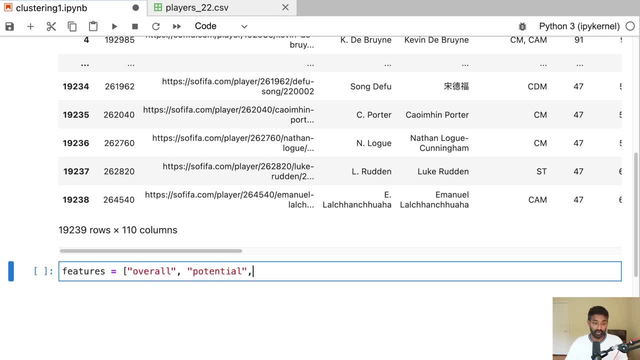 That's going to be overall rating, potential rating, wage: EUR. so the salary value: EUR. so the total value to the club and age. So these are the features that we're going to use to cluster our players based on, And then what we're going to do is we're going to use the 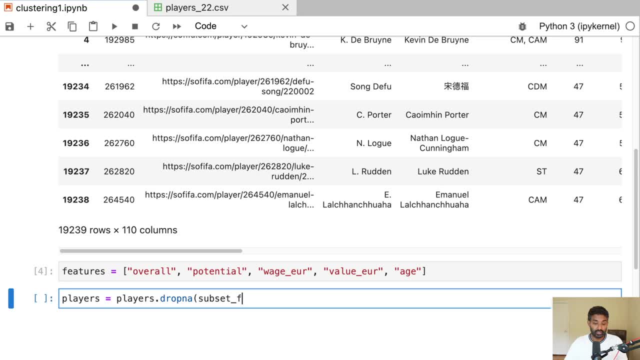 drop na method in pandas to drop any rows where one of these columns has a null or missing value. That's what this subset parameter does. It says: look at these five columns and if there is a null or missing value, just drop the row. 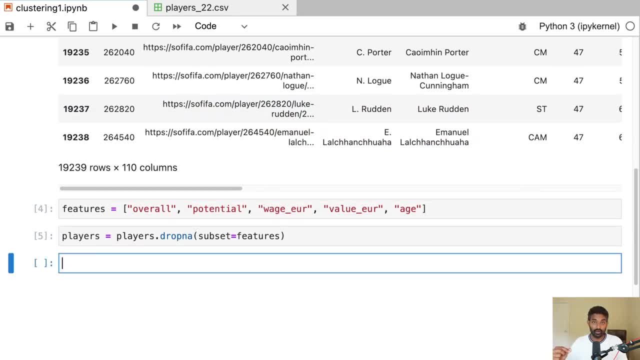 This makes sure that we don't have any missing values in what we're going to be clustering. Most clustering algorithms aren't able to work with missing values, so this just ensures that the data is properly set up for clustering. Then we're just going to copy some of our player data. 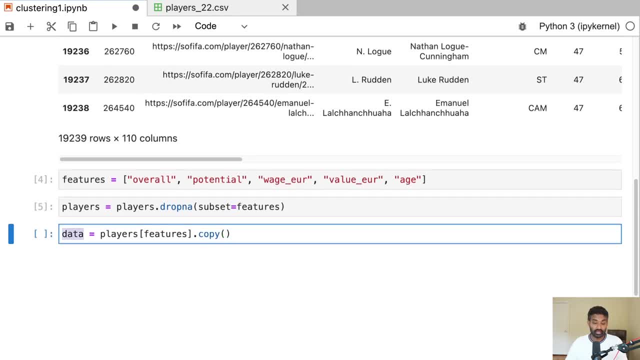 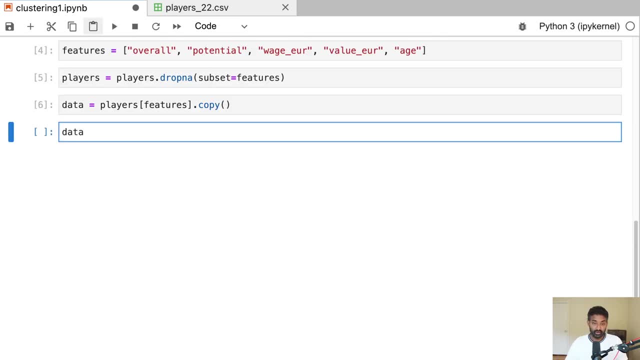 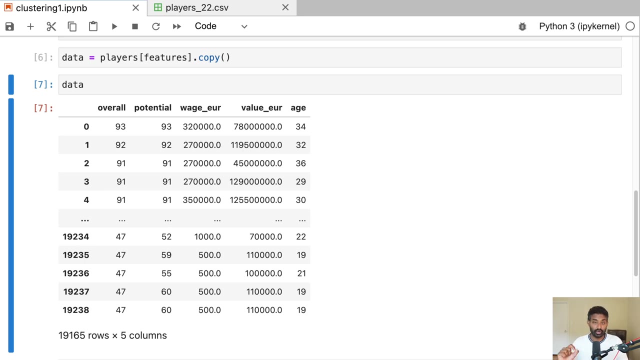 into a new data frame, and this data data frame is what we're going to use to actually do our clustering. All right, So if we look at data now, we can see it only has the five columns that we care about and, given this, we can actually go ahead and start implementing our k-means clustering. 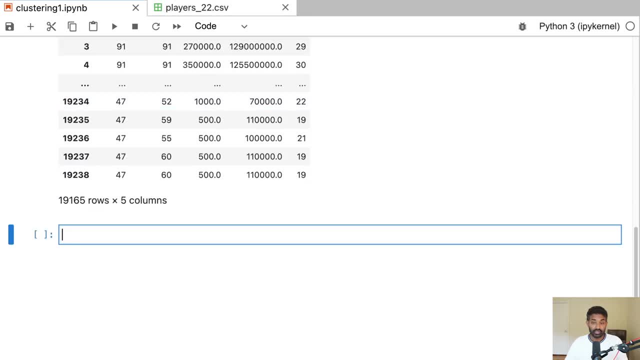 algorithm. So the steps we're going to use to do our k-means clustering, I'm just going to briefly write out so that we can come back to them and see if we can do them in a better way. So let's do a. 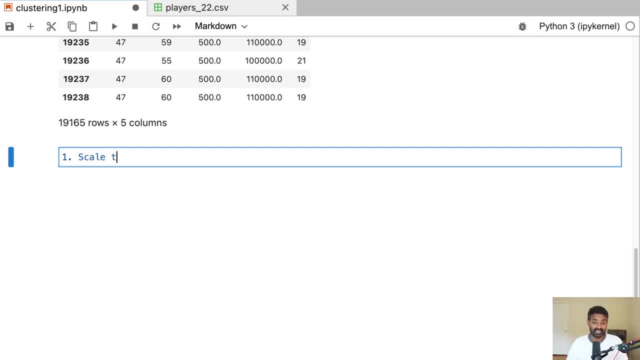 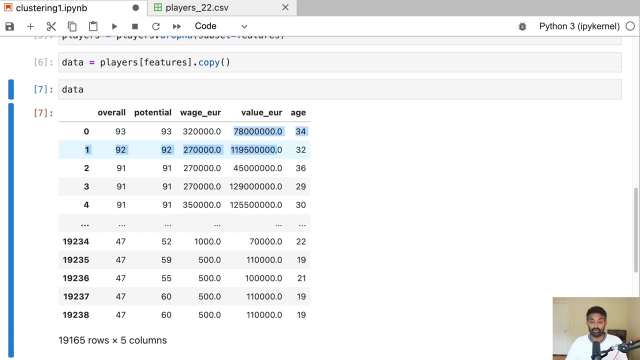 to them and refer to them. so the first thing we want to do is scale the data. so what this means is we want the data to go from a certain value to a certain value. so if you look at our data here, some of the columns have values that are much larger than values in other columns. so when we 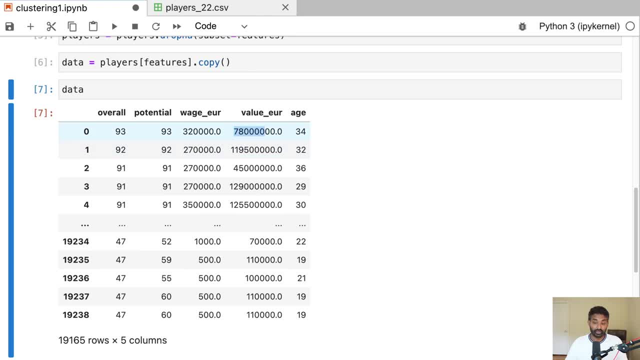 do our clustering. these columns with the largest values will have the most importance in our clustering, but that's not necessarily what we want, right? we want every column to be treated equally when it comes to doing the clustering, so we're going to rescale the maximum and minimum. 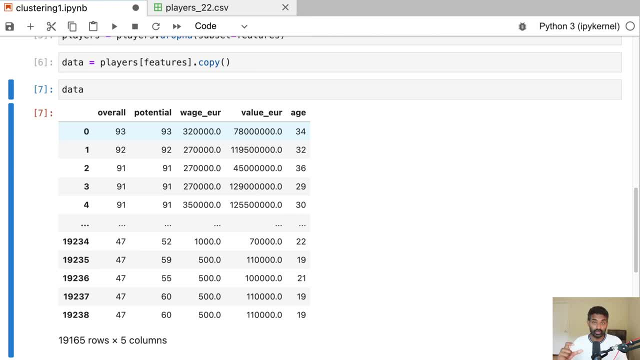 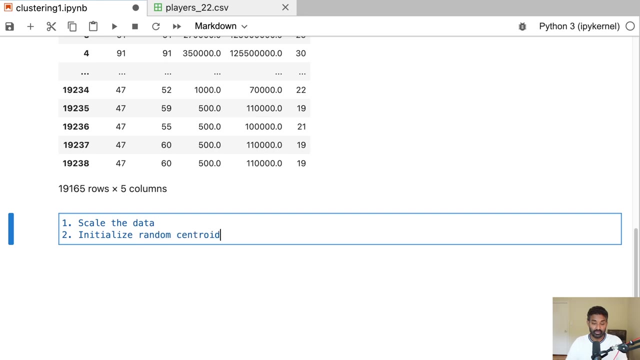 value in each column, so that all the values are in the range 1 to 10.. and what this will help us do is it will ensure that no one column dominates the others in the clustering. so that's scaling the data. then we initialize random centroids. so we talked about this earlier. 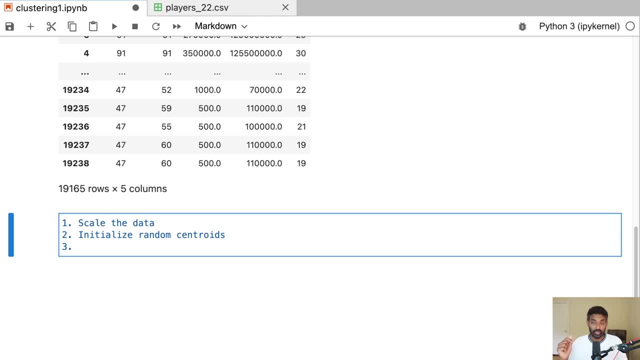 when you create a clustering, you want to make sure that all the values in the clustering are in the range 1 to 10, and so when you create and start your k-means algorithm, you initialize random centroids at first. then we're going to label each data point based on how far that data 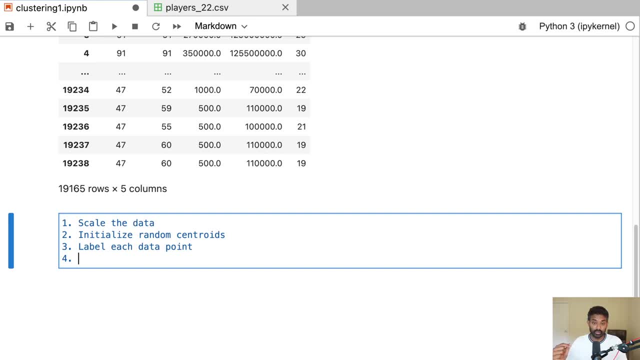 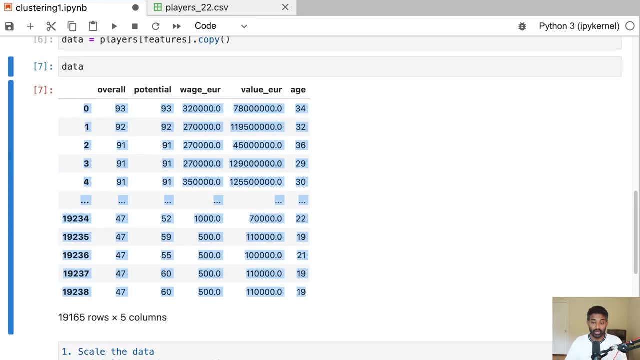 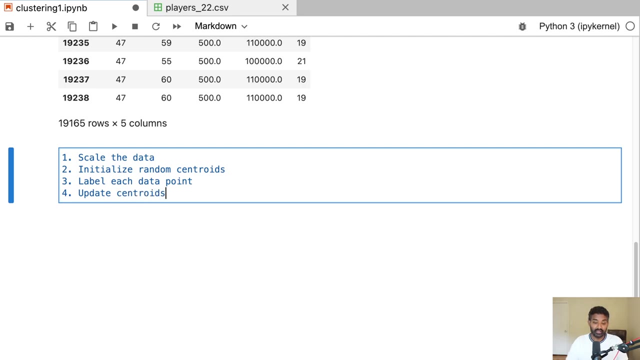 point is from each centroid, so that will give us our cluster assignment for each football player. each data point is one row in our in our data and each row corresponds to a football player. then we're going to update our centroids so we'll look at each player and we'll look at their. 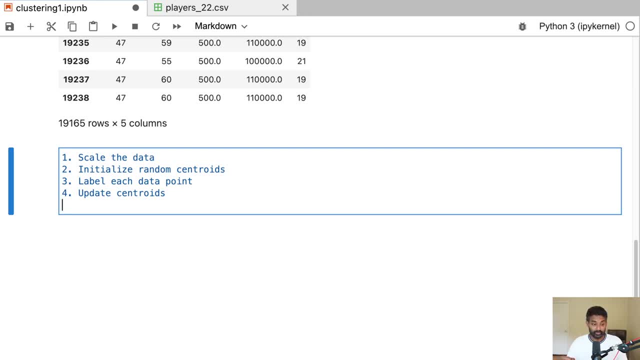 label and then we will find the center point of each cluster and then we're going to repeat steps 3 and 4 until centroids stop changing. so we'll wait till the algorithm converges and gives us our final cluster assignments. so this, at a high level, is the steps that we're going to follow. so the first thing we're going- 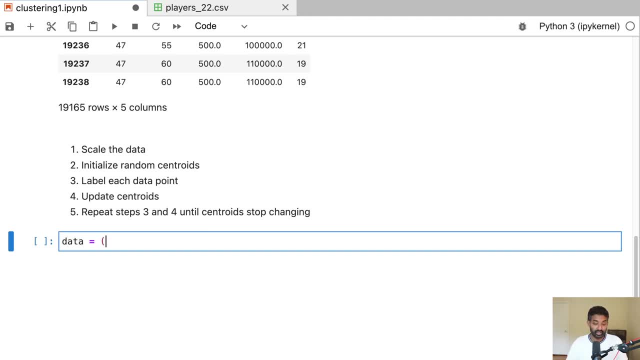 to do is scale our data, and we're going to use something called min max scaling. so the first is we'll subtract the minimum value in each column from each value in the column, And what that does is it sets the minimum value in each column to zero. 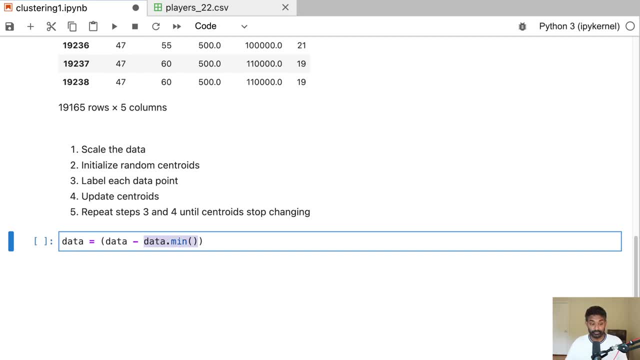 because we're subtracting the minimum value from each item. Then we're going to divide by the range, So datamax minus datamin. So what this does is it rescales everything from zero to one. Then we're going to multiply it by nine. 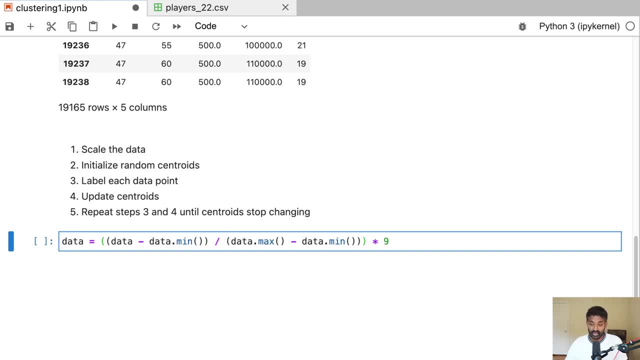 And what this will do is rescale everything from zero to nine And then we'll just add one so that everything is on a one to 10 scale. You can definitely do a different scale If you want to do a zero to one scale. 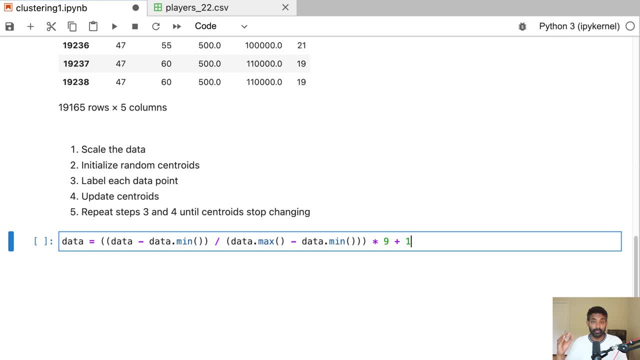 or even a one to a hundred scale. that will work out. Actually, you don't want to do a zero to a 10 scale. You basically don't want a zero or a negative scale. You want a zero or a negative value in your scale. 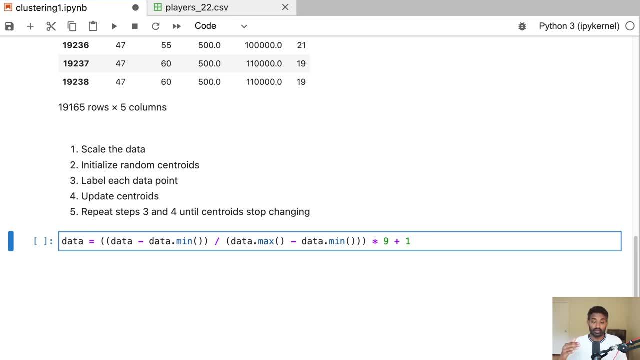 So your minimum needs to be greater than zero, And other than that, you can feel free to do whatever scale feels comfortable to you. And then what we can do now is we can say datadescribe, And what we'll see is that our minimum value in each column is a one. 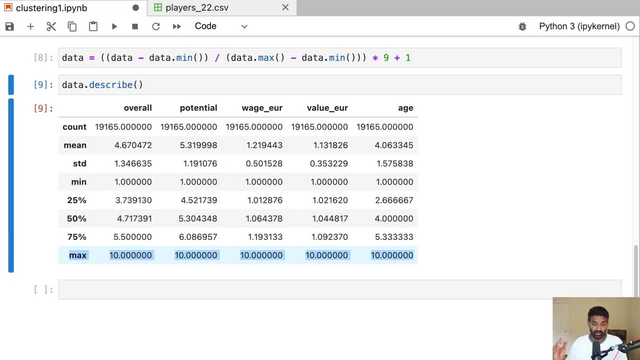 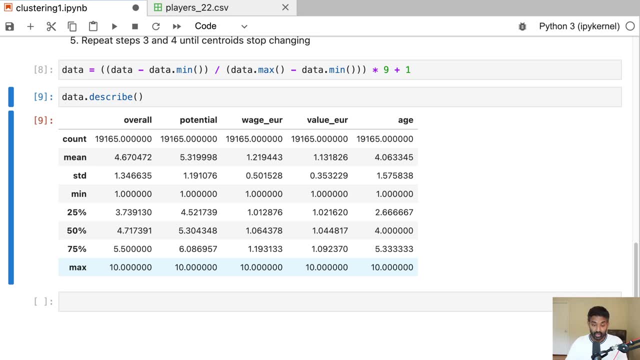 and our maximum value in each column is a 10.. So everything is now on a one to 10 scale, which means that no one column will dominate the others in the cluster. We've also preserved the minimum value in each column. We've also preserved the variance in our original data. 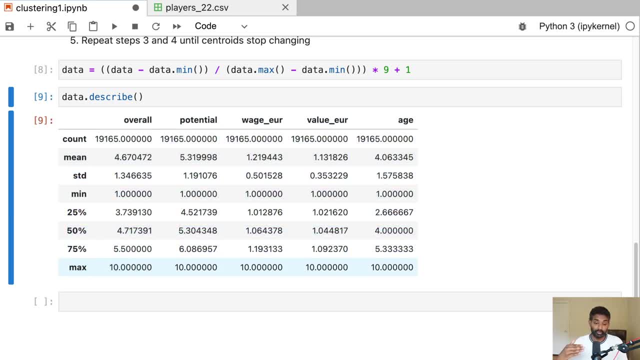 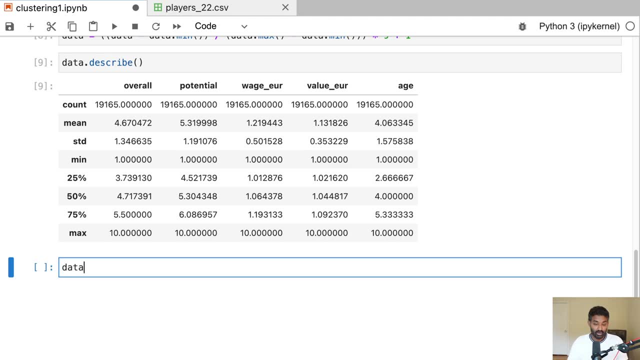 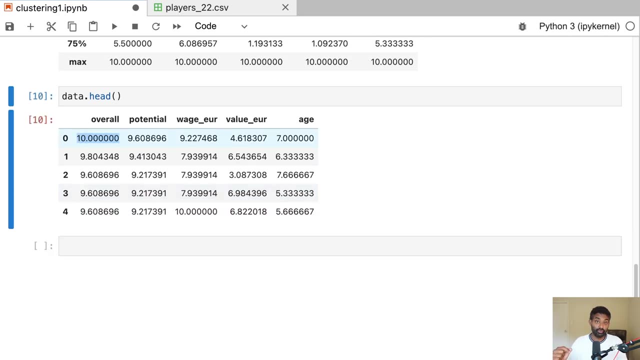 So, if one player had a much higher potential than another player, that's still preserved in our data And that's what we want to preserve. All right, let's take a look at the first few rows in our data So we can see Lionel Messi has the highest overall rating. 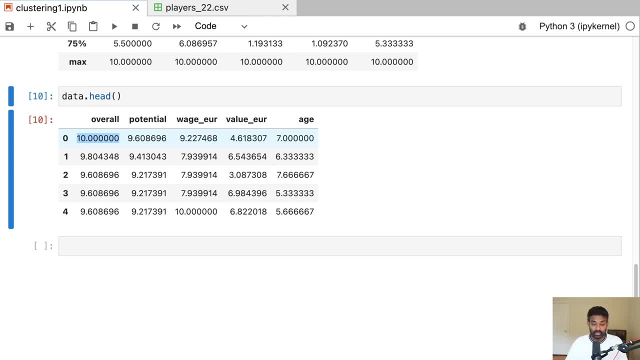 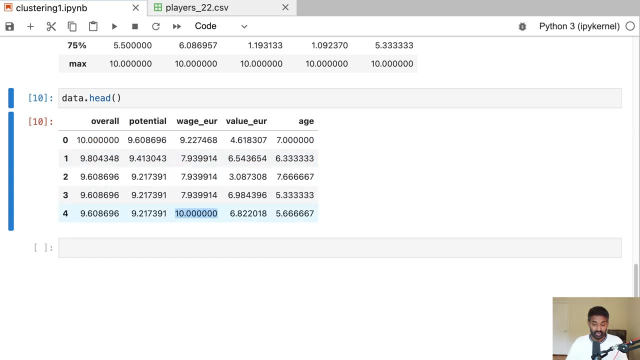 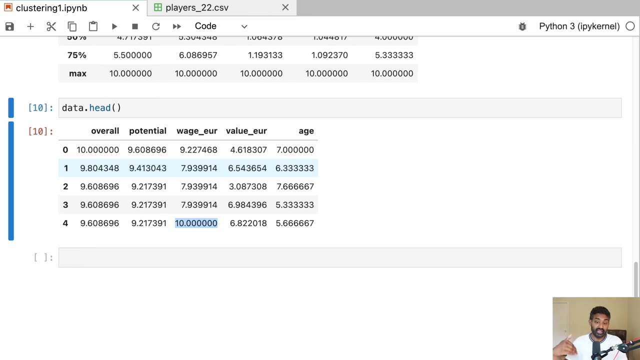 in FIFA out of any player And his rating is now a 10, which is the maximum value that's possible, And then you can see: this player had the highest possible wage, So that shows up as a 10.. And then everything else is scaled down. 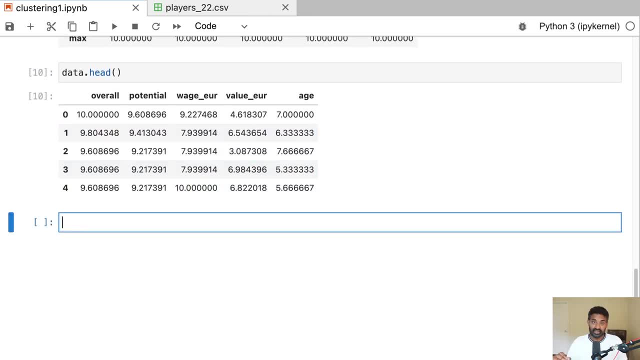 according to the min and the max. All right, so we've loaded our data in and we've processed it and scaled it properly. So the next thing we need to do is initialize our random centroids. So to do that, we need to create, essentially, a value for each feature. 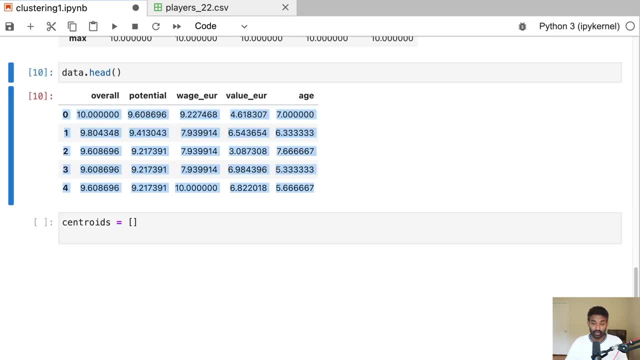 So a centroid is just going to be similar to a row here. it's going to have a value for each feature, for overall, for potential, for wage, But we need those values to be random from our data set. So what we're going to do is we're going to say: 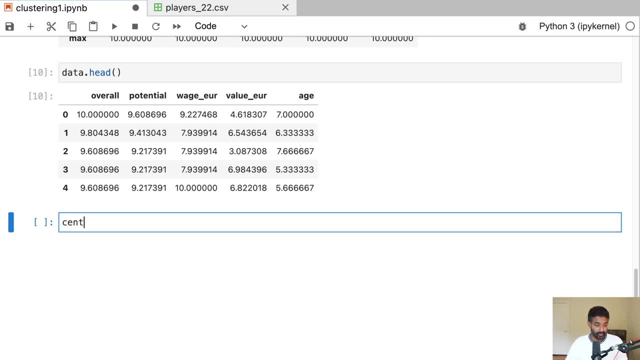 actually, let me get rid of this for now. We're going to say centroid. So if we want to create a single centroid, we're going to say centroid equals dataapply lambda x below to xsamp. So what's this doing? 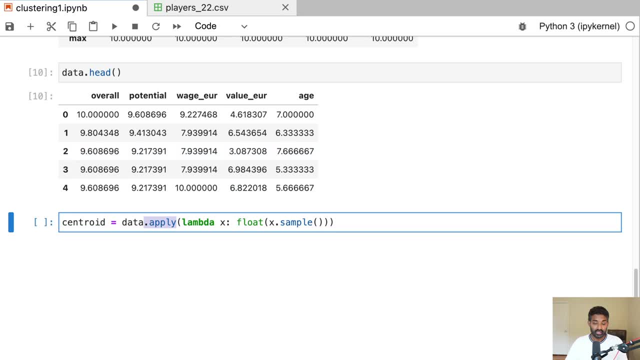 So the apply method on a data frame is going to iterate through each column in the data. So we're going to look through each column So overall, then potential, then wage, And then we're going to call xsample And what that does is it selects a single value. 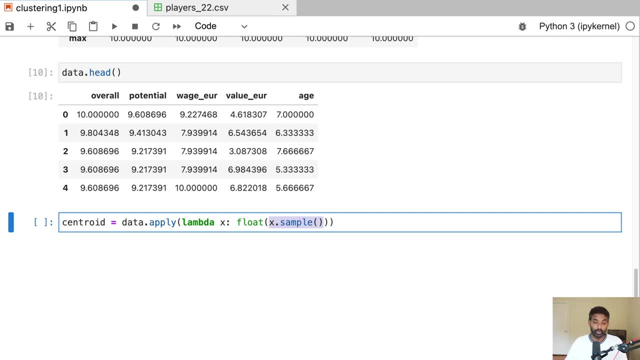 from that column a random value. So we're going to randomly sample a single value from each column And then we're going to turn it into a float, because xsample returns a panda series and we want it to be random. We don't want it to actually be just a single number. 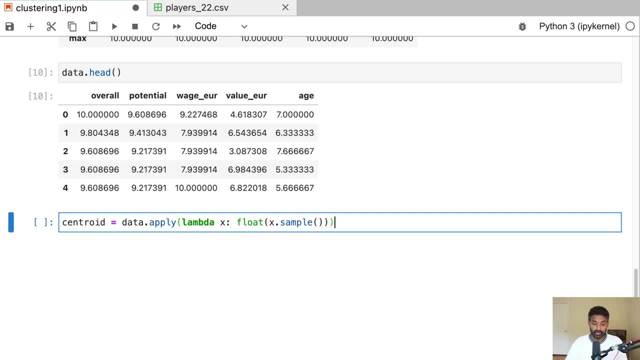 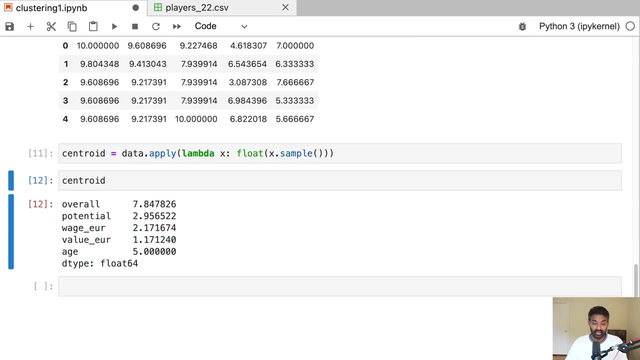 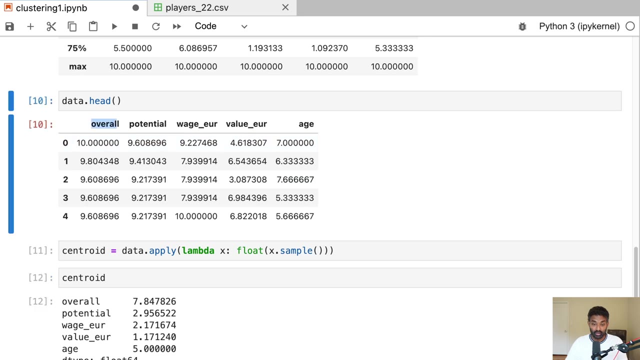 So we then call float to turn it into a number. So if I run this and I look at centroid, centroid is now a panda series and it has a random value. well, randomly sampled from our data value for each column, You could instead just find a random value. 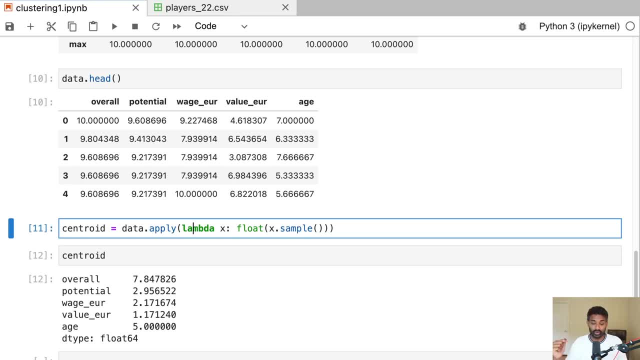 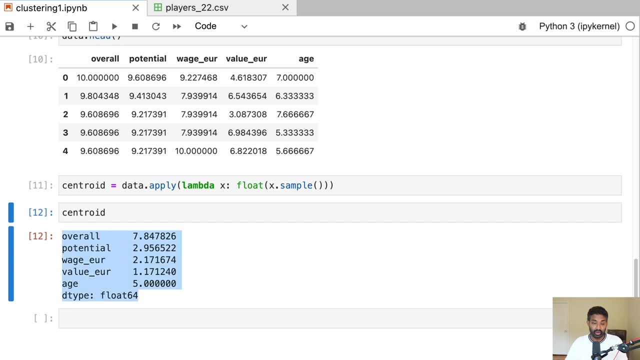 from one to 10 and use that as your centroid also. Also, that's another way that you could initialize these random centroids. So we have a single centroid. Now we need to scale this method up to get multiple centroids. So if we're looking for k clusters, 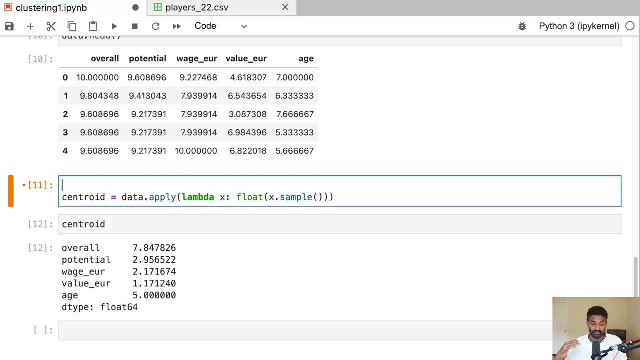 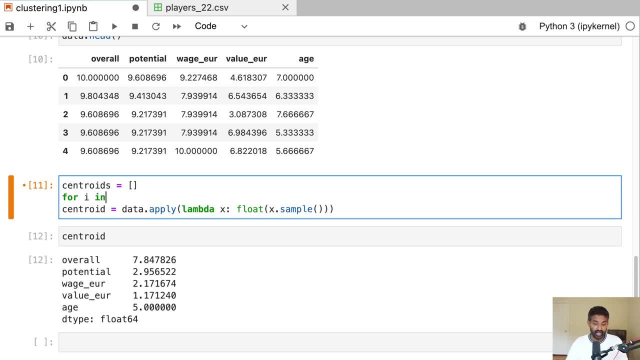 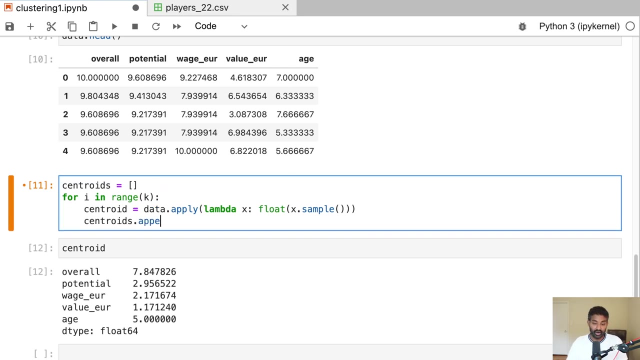 we need k centroids. So if k is five, we want there to be five centroids that we initialize. So we'll initialize a list called centroids and we'll say for i in range k, create the centroid and then add it To our list of centroids. 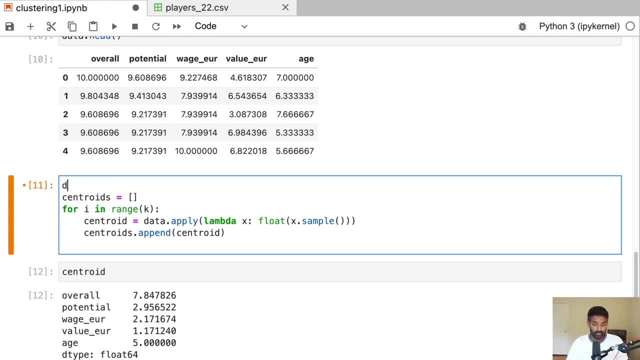 And then we will wrap this into a function, So we'll call a function called random centroids. We'll take in our data and we'll take in the number of clusters that we want. right, If you remember? each centroid is just the center of each cluster. 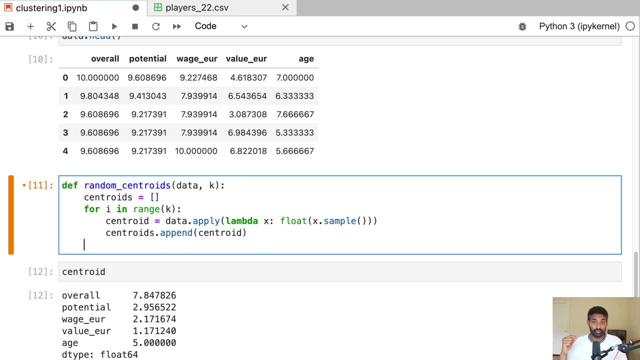 So the number of centroids we create is equivalent to the number of clusters we want, And then what we'll do is we'll return pdcloncat centroids. x is equals one. So what this does is it combines all of the individual panda series. 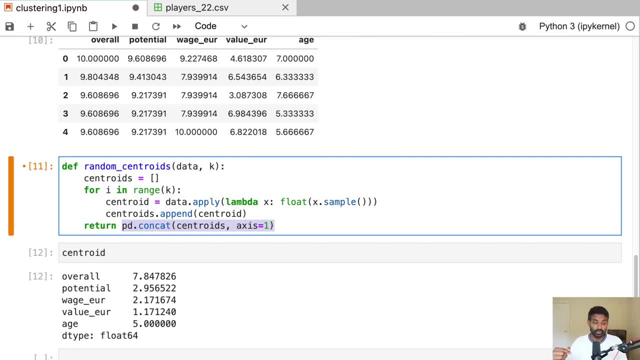 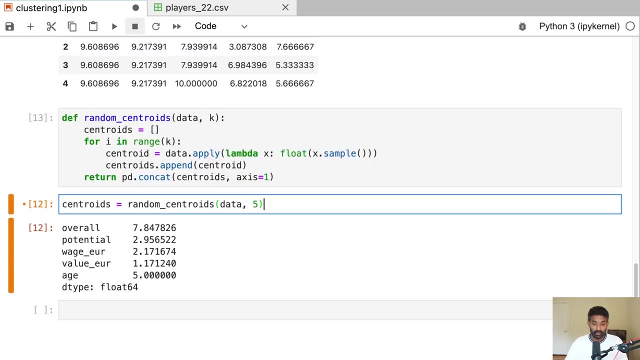 Remember, each centroid is a panda series. It combines all of those individual series into a data frame. So now we can run this to generate our centroids. Let's call random centroids data And let's say we want five clusters. So let's take a look at our randomly initialized centroids here. 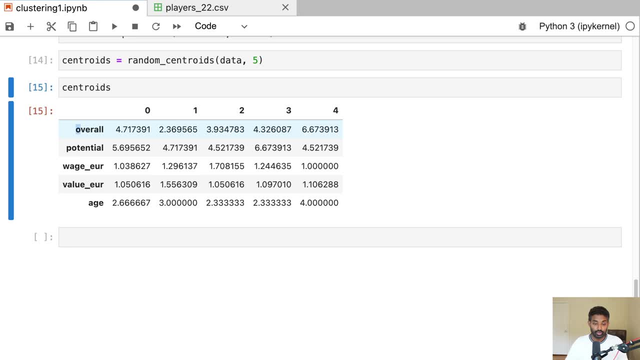 So each centroid is a data frame. So each centroid is a data frame. So each centroid is a data frame. So each column is a centroid And each row is a different feature. So cluster zero, the centroid would have this overall value. 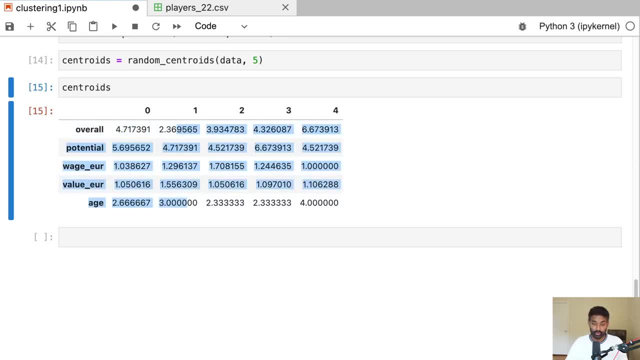 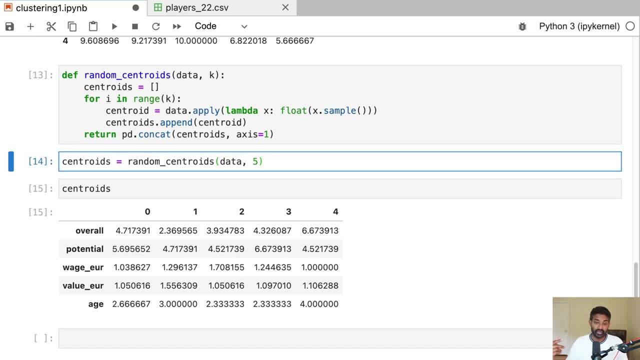 this potential value and so on. Then cluster one, cluster two, cluster three, cluster four also have those values. If you changed k, you would generate a different number of centroids. right? If you only want three clusters, you would only generate three centroids, and so on. 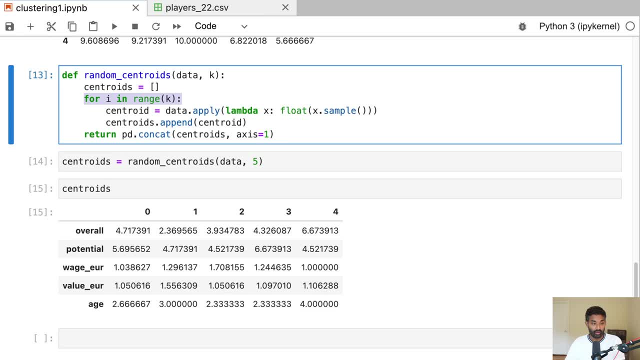 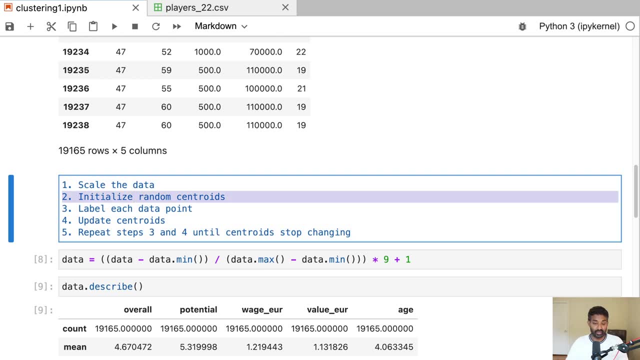 And that's what this loop is doing. So we've completed the first step in our algorithm, or the first two steps. We've scaled the data and we've initialized random centroids. The next thing we need to do is write a function. 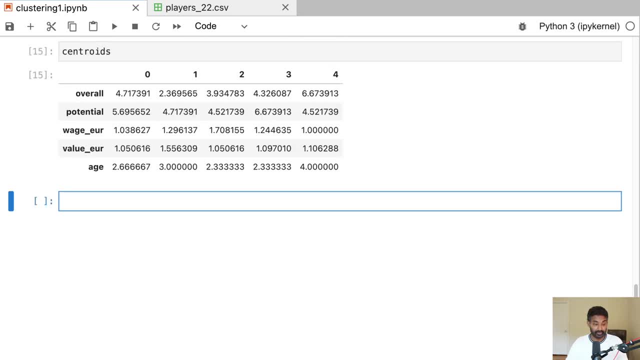 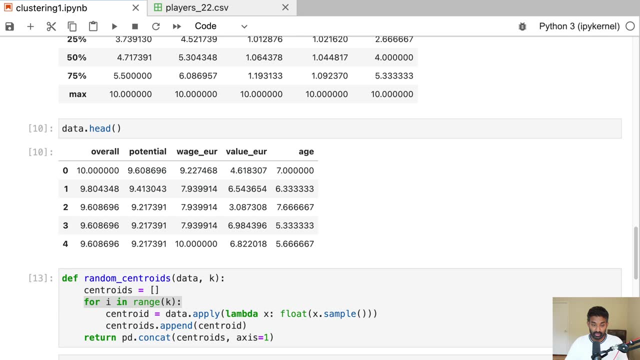 that labels each data point according to the cluster centers, And what this function is going to do is it's going to look at each player in our data, each data point in our data frame, and it's going to find the distance between the Euclidean distance. so geometry. 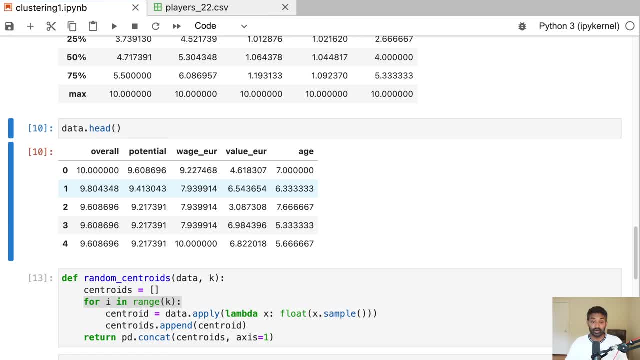 between that data point and each cluster center, And then we're going to find the cluster center that is the closest to that data point. So for this first data point, which represents Lionel Messi, we're going to evaluate the distance between Lionel Messi's 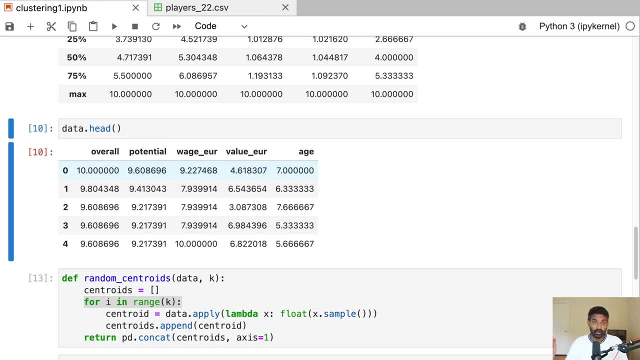 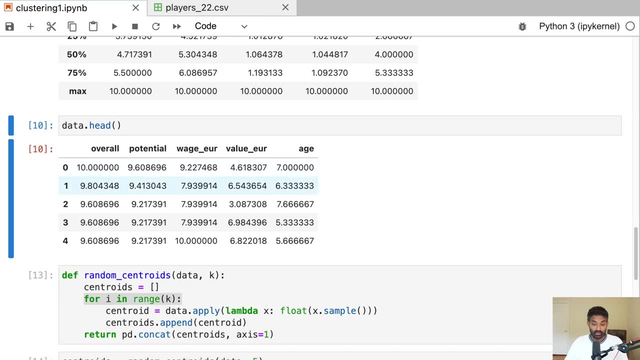 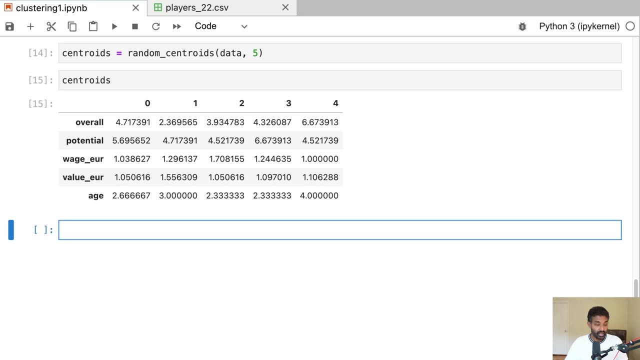 overall rating, potential wage and each centroid, And then we will take the centroid that's the closest and assign Lionel Messi to that cluster. So we will do this by writing some code to calculate the distance. So to calculate the distance, you may be familiar with this formula from geometry. 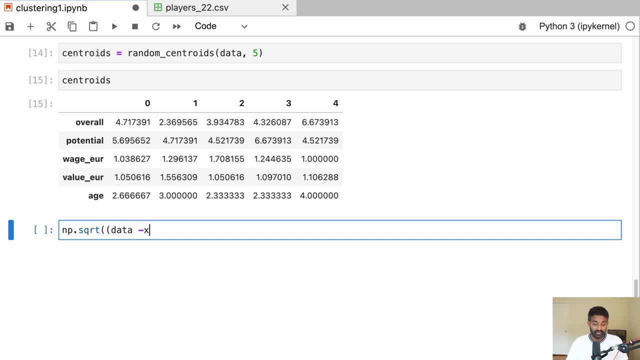 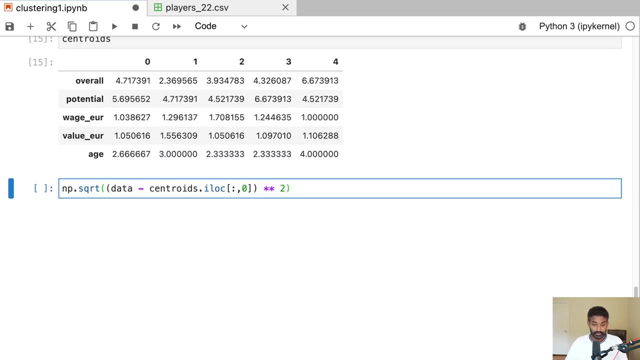 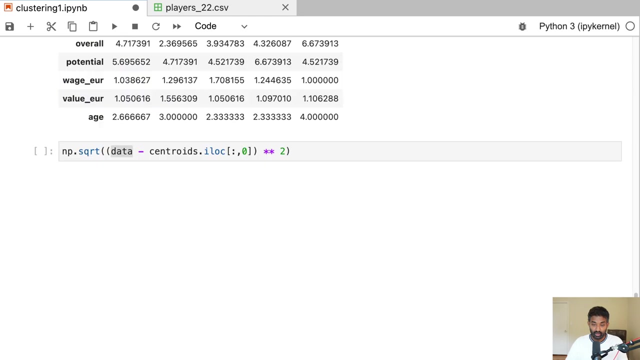 We are going to subtract the centroid, So this will give us the centroid for cluster 0. So we square that and then we take the square root. So we subtract the values for the centroid from each data point. Then we square that. 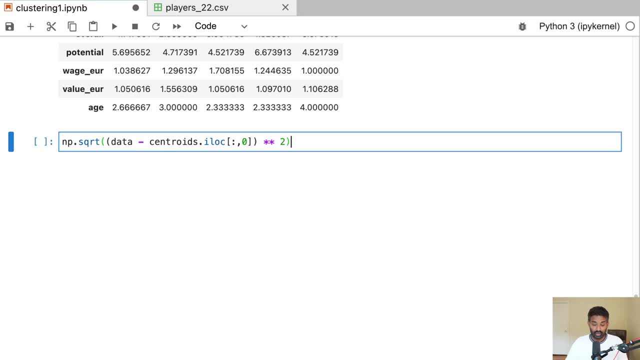 and then we take the square root of the overall result And that is a distance formula from geometry. And then Right. okay, So inside here- Sorry, I missed a parenthesis- We want to add all the distances up before we take the square root. 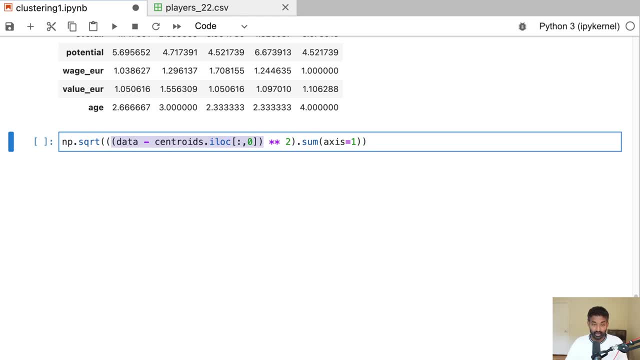 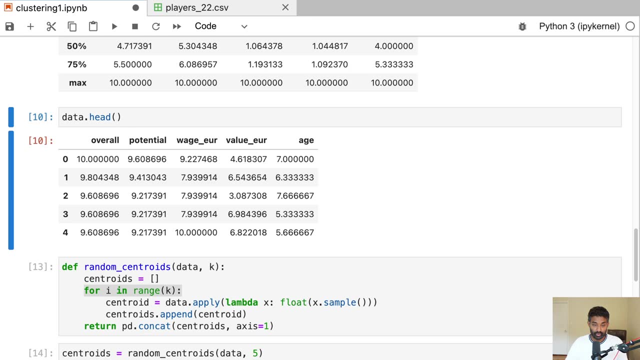 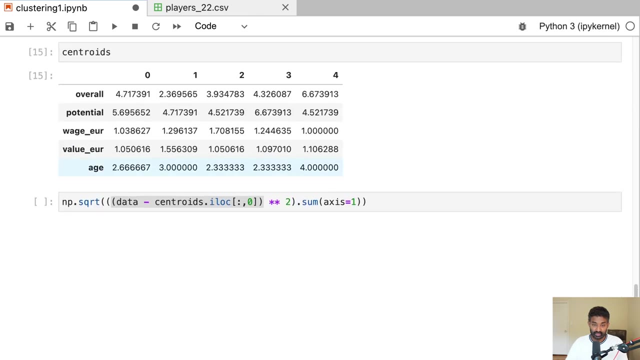 Okay. so what we're doing here is we are subtracting from our, From our, From each row we're going to subtract the values for the centroid. So we do overall minus the overall value for centroid 0. We do potential minus the value for centroid 0, and so on. 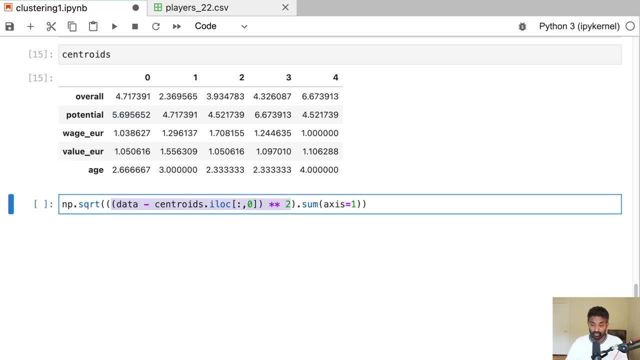 And then we would square each difference. We would add all the differences together and then take a square root which is just a distance formula, And then what we are going to do. these parentheses are tricky. I need to make sure. I'll make sure they're all in the correct place. 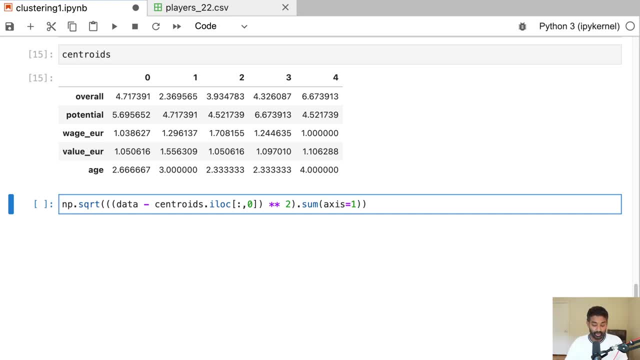 Otherwise the formula is going to be incorrect. Then what we'll do is we will apply this to all of our centroids. So we'll say centroidsapply lambda x And then we'll replace this with x. So what this will do is it will apply this function. 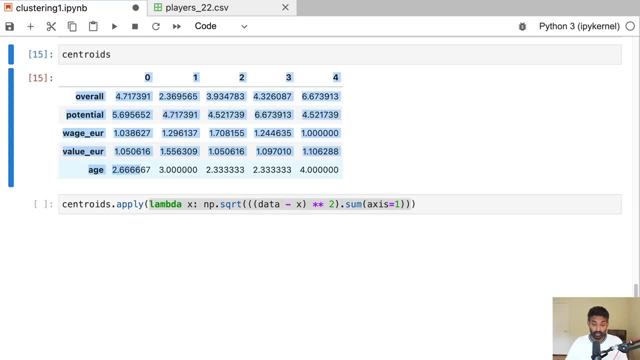 to each of our centroids, Because each centroid is a column and this is going to apply a function to each column And we can assign the result to a variable called distances. So let's take a look and see what what distances is. 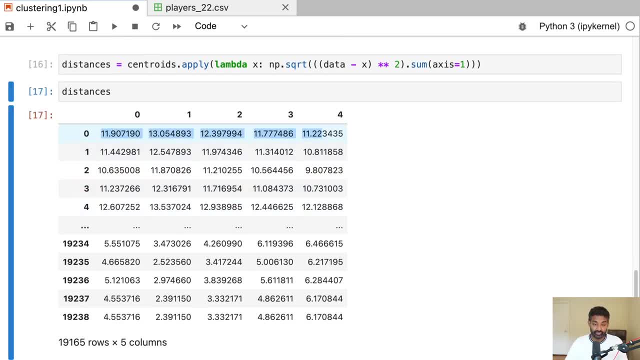 So this gives us a number that represents the distance from each player to each cluster centroid. So this first row would represent This first value here, represents the distance from Lionel Messi to the center of cluster 0. And we can see here the closest cluster to him. 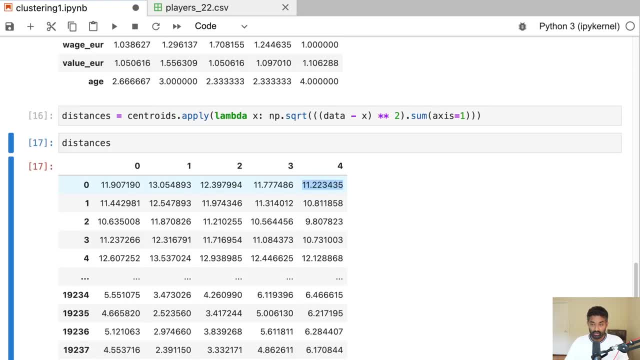 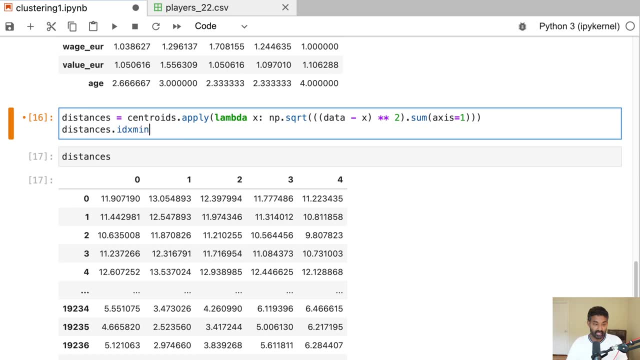 is actually cluster 4, because it has the least distance. So the next thing we need to do is automatically figure out which cluster people are in, And we can do that by doing: distancesidxmin axis equals 1.. So this finds the index of the minimum value in each row. 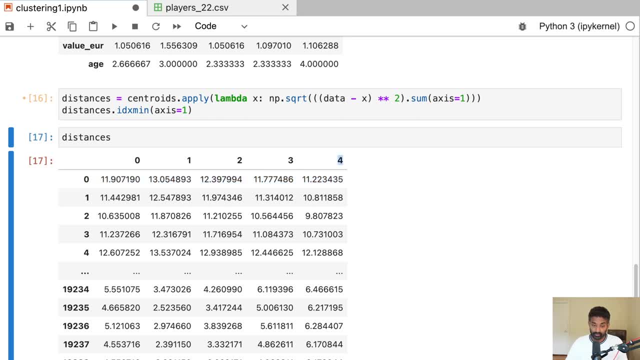 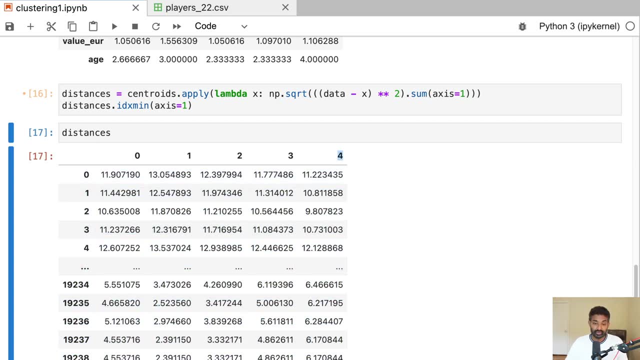 So the index of the minimum value in this row is 4.. The index of the minimum value in this row is also 4.. And you can see the index of the minimum value is also the cluster assignment. So this will tell us which cluster each player should be in. 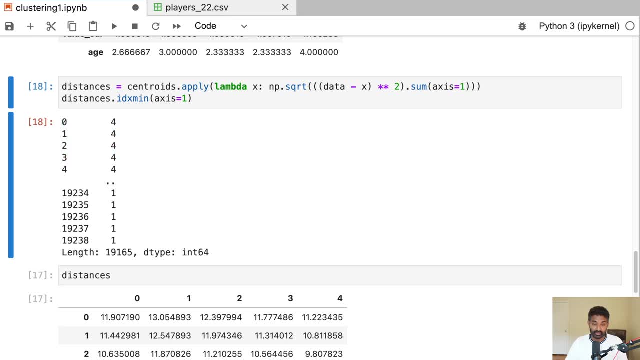 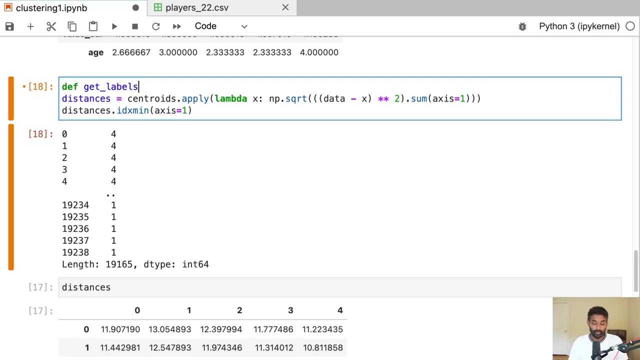 So we can see we now have the cluster assignments for each player And then we'll wrap this into a function called getLabels And we'll pass data and centroids into this function And then we will return this piece, the label. So this is calculating the distance. 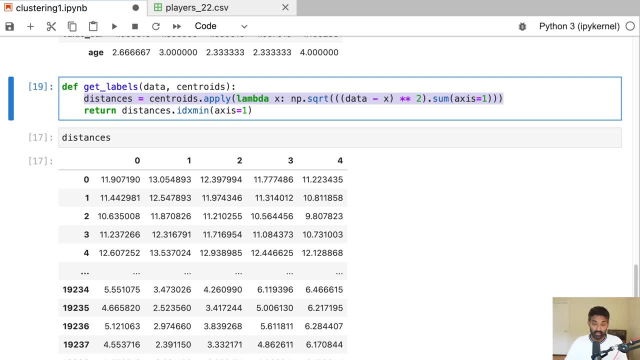 between each centroid and each data point, And then this is finding the cluster assignment for each data point, And each data point is just a player. So it's finding the cluster assignment for each player. So that's getLabels. And then what we can say is: 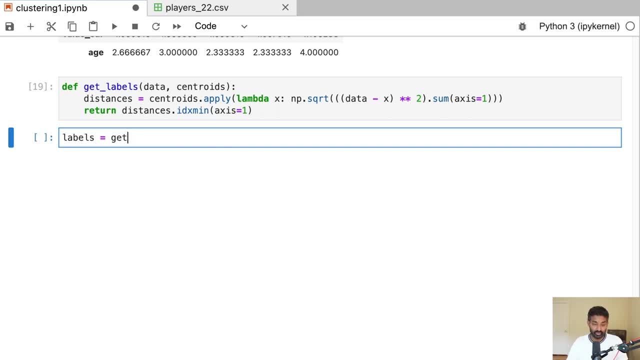 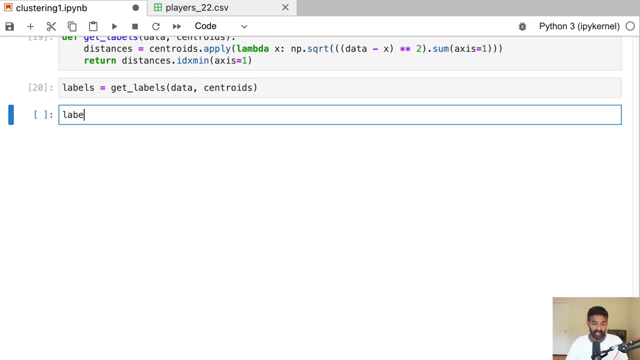 we can just write some code to say: labels equals, getLabels, data centroids, And this will return the same thing. we just saw the labels for each player, The cluster label, rather for each player, And then we can see how many players are in each cluster. 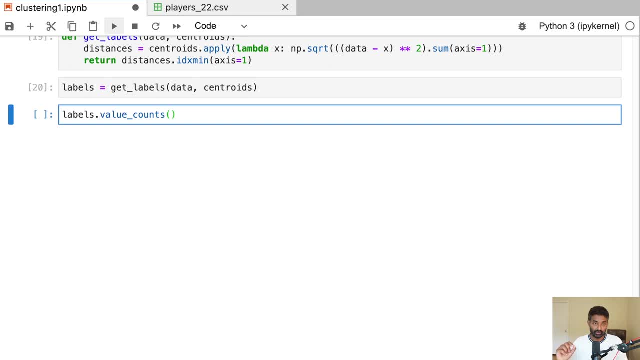 by looking at labelsvalueCounts: So valueCountsvalueCounts, So valueCountsvalueCounts, So valueCountsvalueCounts, So we can count up how many times each unique value occurs in a column. So we can see: 7,600 players are assigned to cluster four. 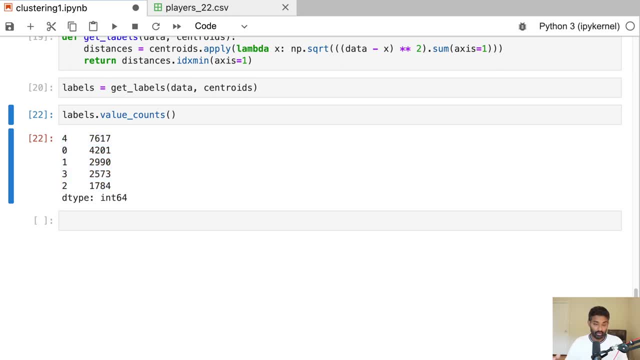 and so on. Okay, so we've now assigned each player to a cluster based on our random centroids. The next step is to actually update the centroids based on who's in the cluster. So what we want to do is find all the players in a cluster. 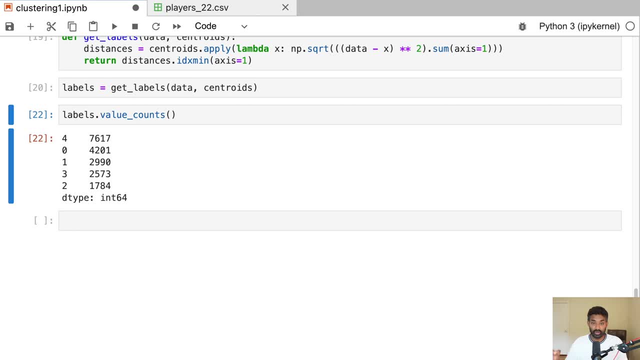 and then take the geometric mean of each feature. So the geometric mean is a little bit different from the mean you're probably familiar with. The mean most of us are familiar with is the mean where you add a bunch of numbers together and then divide by the count. 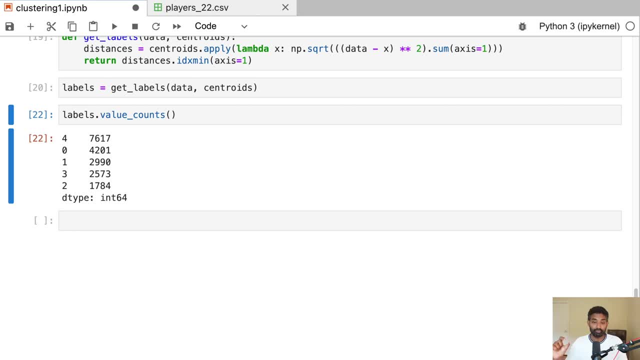 We're going to take the geometric mean, which is the mean of points, the center of points in Euclidean space, And what this gives you is the center of each cluster. So you find the geometric mean by multiplying each point together and taking the nth root. 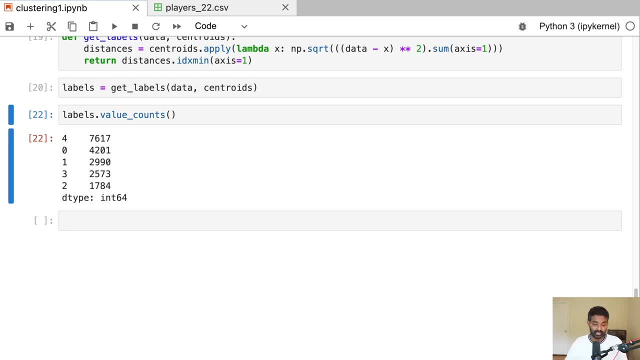 based on the number of points. We're going to do a small modification to how we calculate the geometric mean, so that we don't have to multiply a lot of large numbers together and just get a huge result that takes a lot of memory to store. 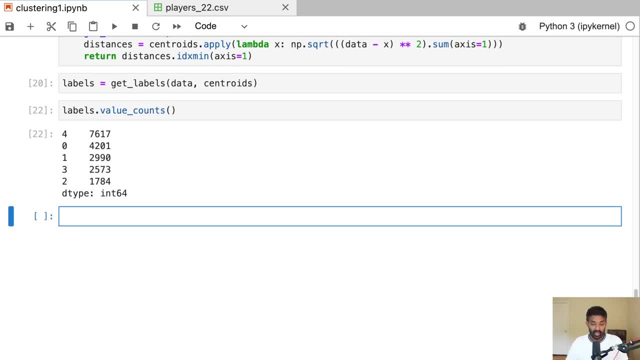 So what we're going to do instead is we're going to say npexp- exp is e to a certain power. Then we'll take nplog, which is the natural log, and then the mean. So what this does is it takes the natural log. 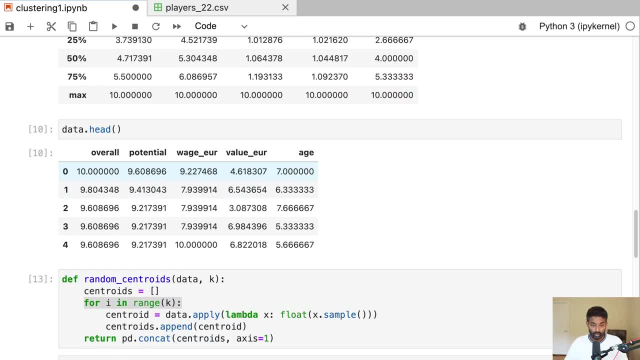 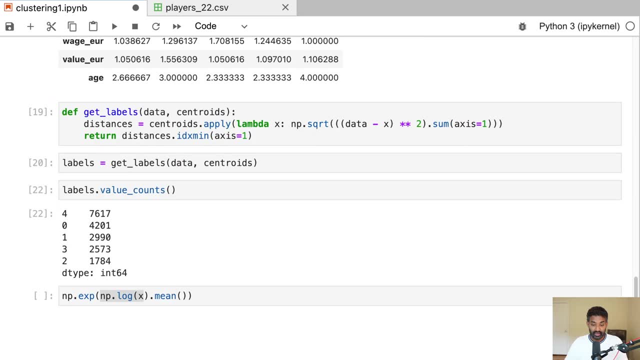 of each data point. So it's going to take the natural log of, for example, each of these values in a given row for a given player. Then it's going to find the mean of all of the values in a row And then it's going to do e to that value. 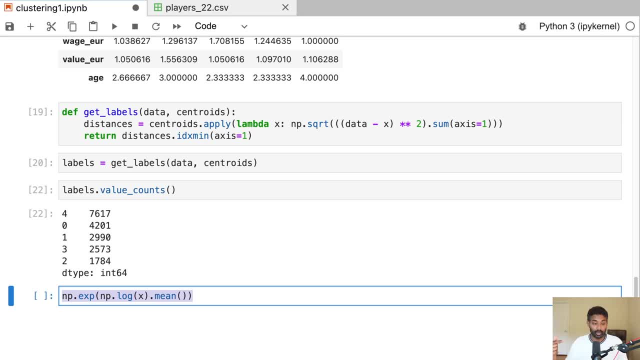 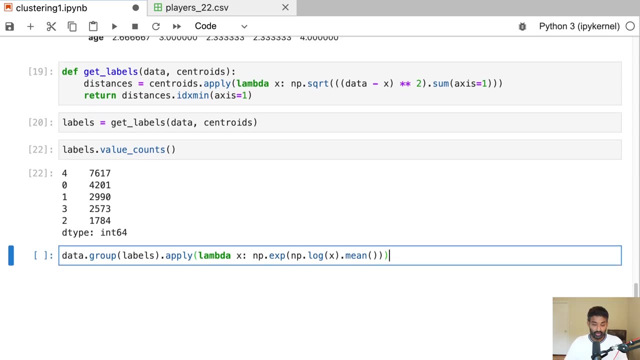 to give us back a result And that's going to be the geometric mean, And then we'll apply this to each of our labels. So we'll say: datagroupByLabelsapply, lambda x is this. So this splits our data up by label. 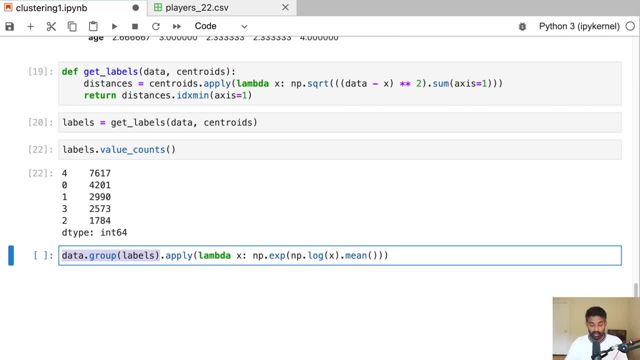 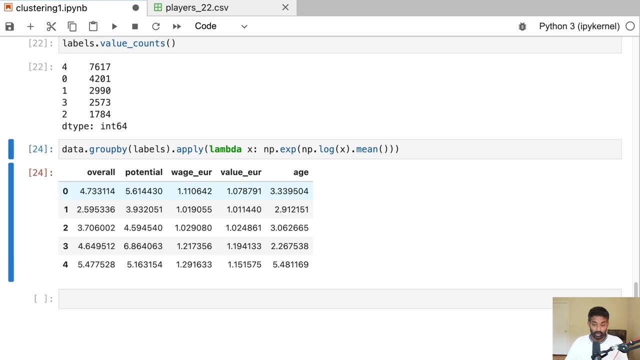 So we create one group for each cluster, essentially, And then to each of those groups we're going to apply this, which will calculate the new centers for each column GroupBy instead of group. Let's run that Okay, and what we end up with is our centroids are in each row. 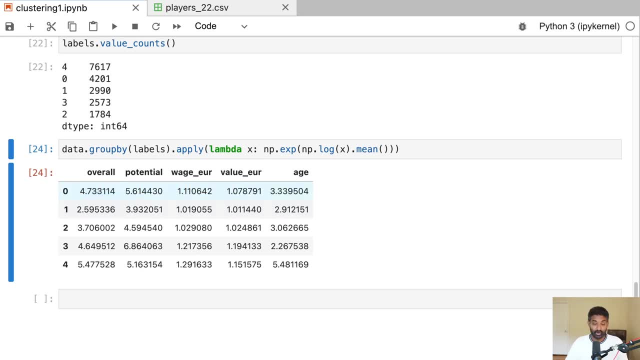 So this is the geometric mean of all of the values, all of the overall values for players who are assigned in cluster 0.. This is the geometric mean for all of the overall values for players assigned to cluster 1, and so on. So the next thing we need to do is 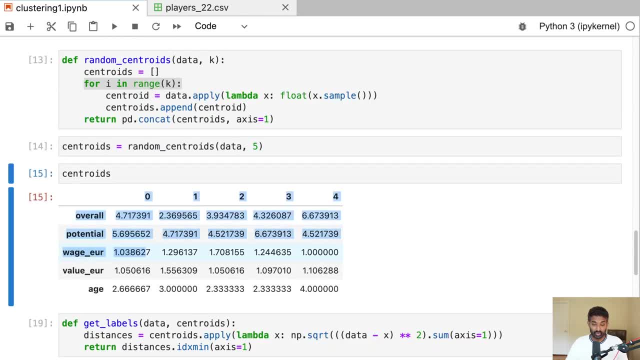 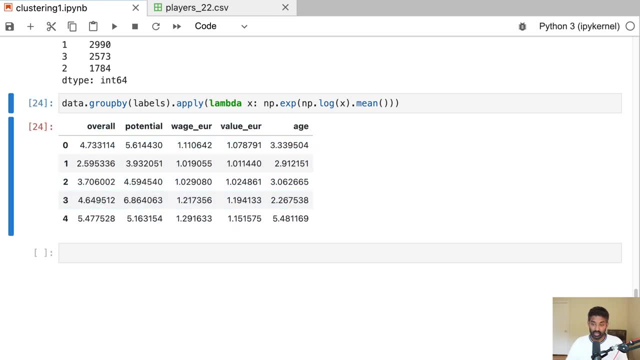 if you remember our centroids from earlier, the columns were actually the centroids and the rows were the features. But here the columns are the features and the rows are the centroids. So we just need to call t to actually turn our data frame. 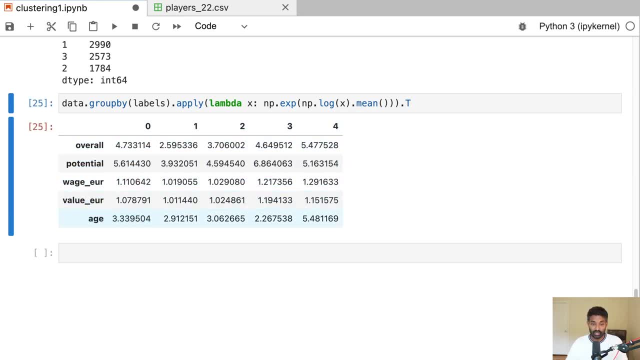 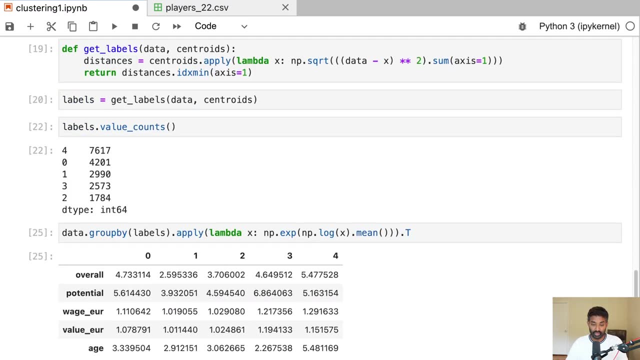 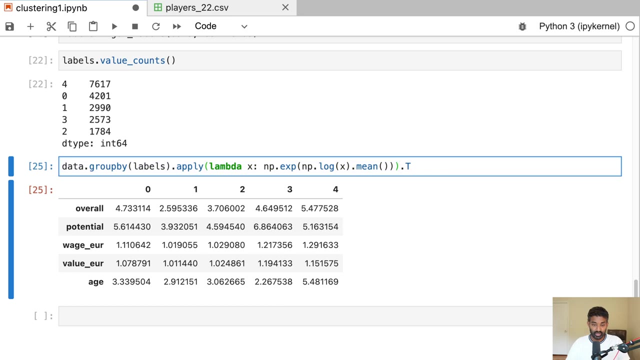 And what that does is now each column is a centroid and each row is a feature, which is similar to what the output of our random centroids function is. Okay, so this may have been a little bit complicated, So let me just explain it one more time. 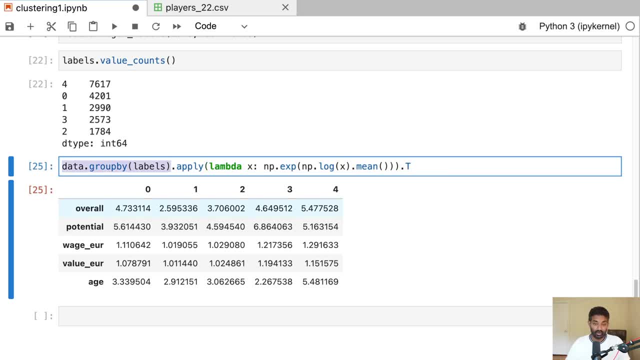 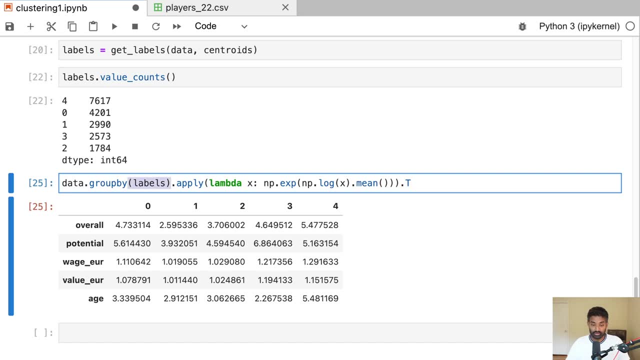 The first thing we're doing is we're splitting our data frame, our data data frame, which contains our player data. we're splitting it up by cluster. So each the labels, the labels series, gives us the cluster assignments. So we're splitting up data by the labels. 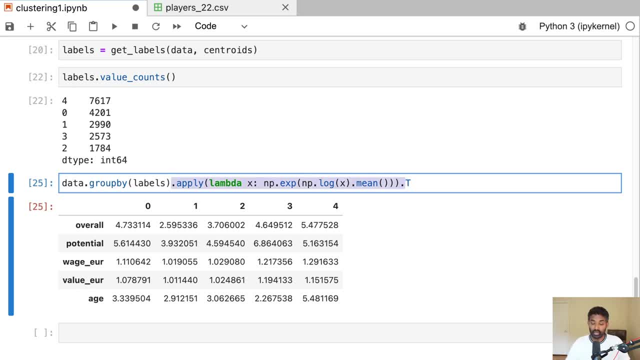 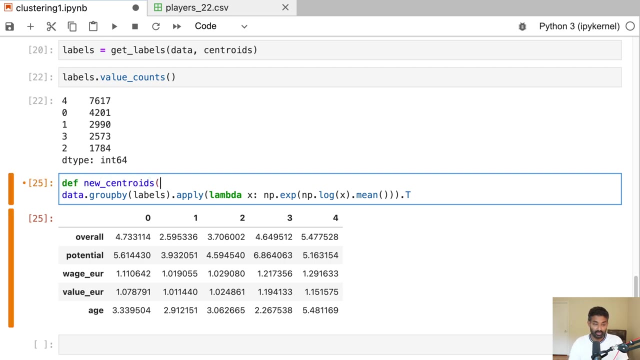 And then to each group we're applying this function which calculates the geometric mean of each feature, And the geometric mean of each feature is the cluster centroid. So it gives us the new centroids. So let's wrap this into a function And we'll run that. 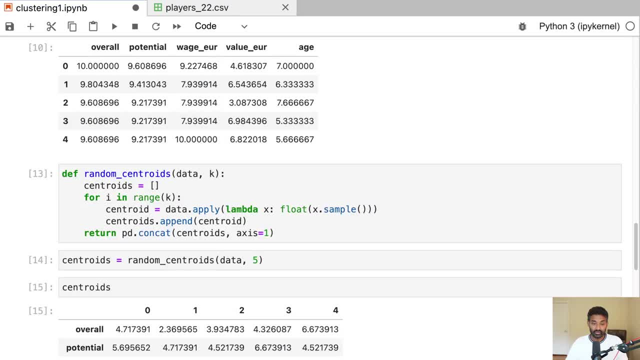 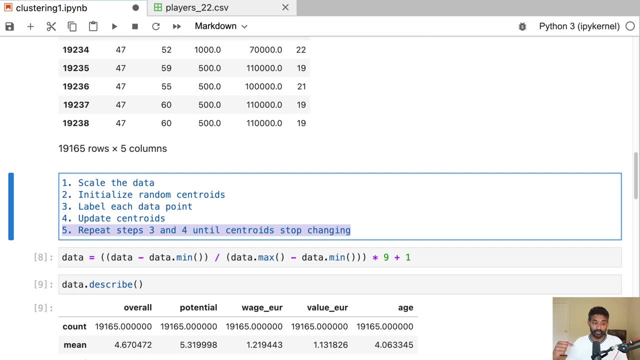 Okay, so we now have all of the pieces. we need to go ahead and write our loop, And our loop will actually make all of this work together and it'll go through our iterations. Now, one thing we want to do. this isn't necessary, but it's very nice to have. 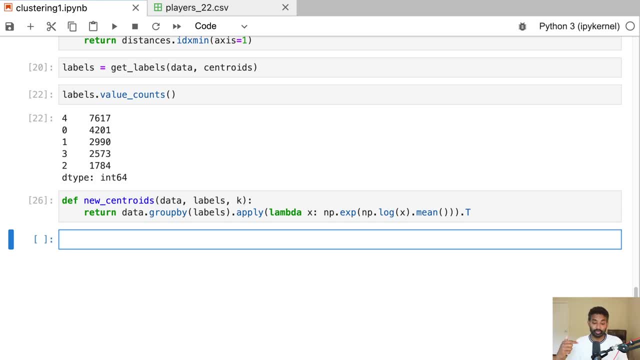 is actually visualize what's happening as our loop, as we iterate in the algorithm and as the loop continues. So we're going to go ahead and write our loop And we're going to go ahead and write our loop And we're going to go ahead and write our loop. 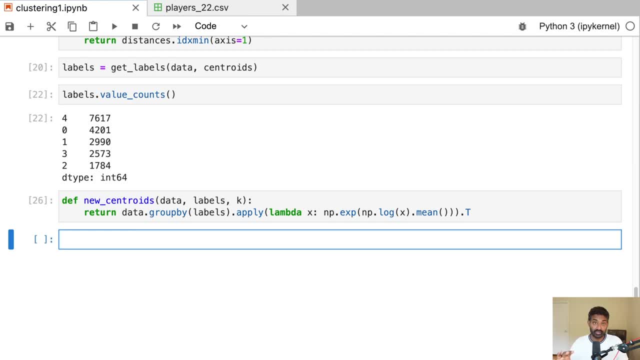 And we're going to go ahead and write our loop. So we're going to write a quick function to actually plot the cluster assignments at each step in our algorithm, at each iteration, And to do that we're going to need to import a couple of things. 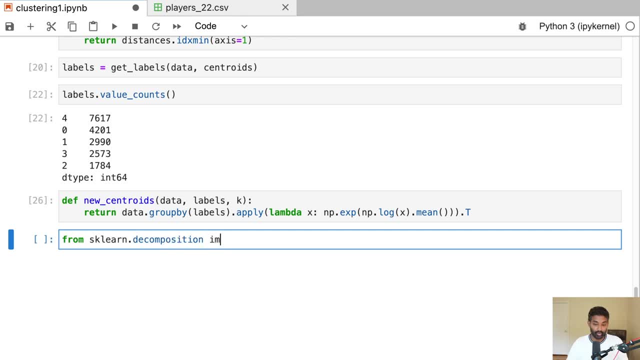 So from sklearndecomposition we're going to import PCA, And then we're going to import matplotlib, Plotlibpyplot, as PLT And then we are going to say: from ipythondisplay, import clear output. So PCA stands for principal components analysis. 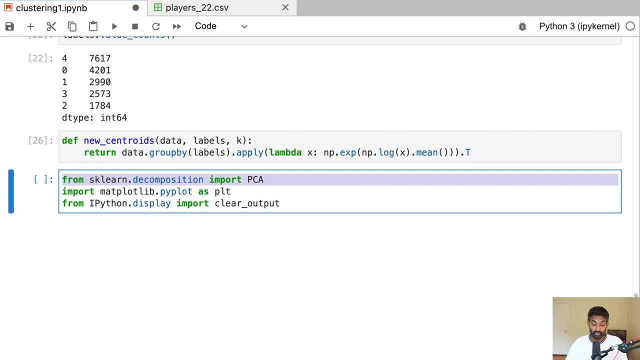 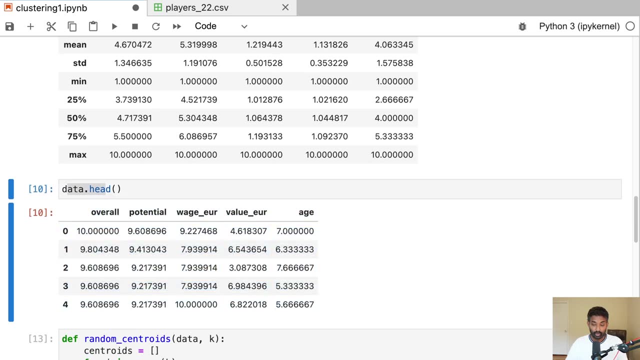 And what it's going to help us do is visualize our data, Because we have five-dimensional data. So our data, if we scroll up and look at our data data frame, we have five features for each player. You can only visualize easily two-dimensional data. 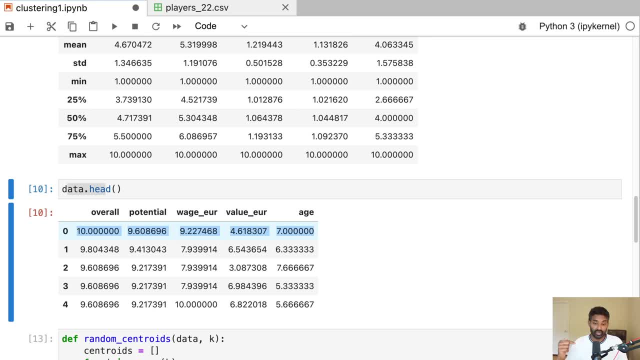 You can also visualize three-dimensional data, but it's a lot easier to visualize two-dimensional data. So we need a way to turn this five-dimensional data into a five-dimensional data, And PCA will help us do that. It'll look at these five columns and essentially summarize them into two columns. 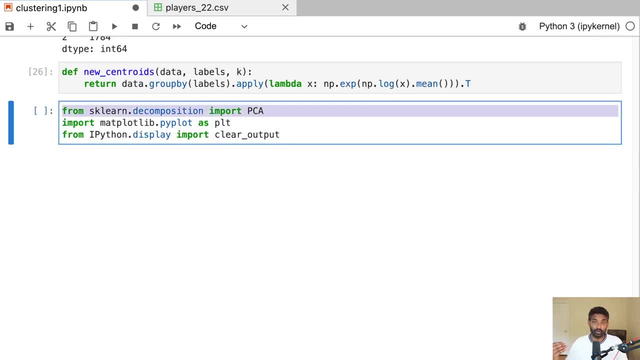 So that's what PCA will do. So this will help us graph our clusters. Then matplotlib will actually do the plotting. So it's a Python plotting and charting library And then this will actually help us clear the Jupyter notebook output each time we plot a new graph. 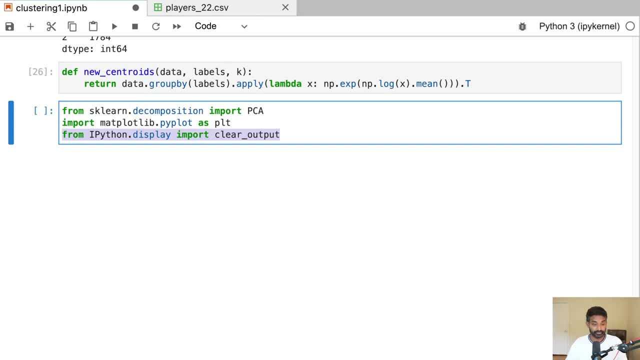 So we clear the output, then put a new graph And then we can go ahead and write our function to plot our clusters. So our function is going to be creatively called plot clusters And we'll take in our data, We'll take in the labels, the centroids and the iteration. 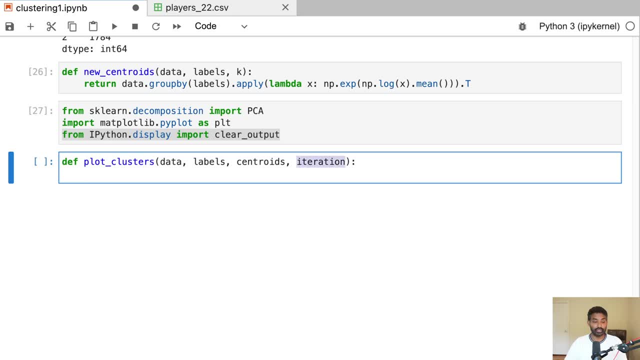 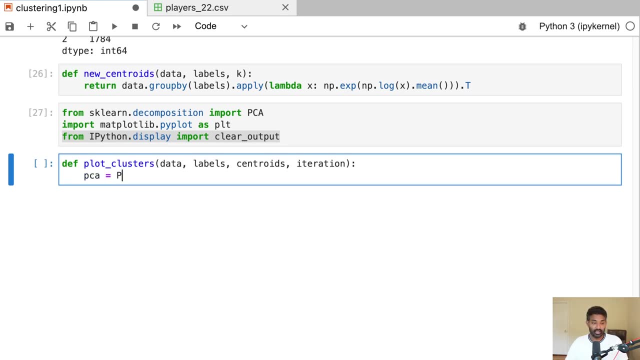 So we haven't done anything with iteration yet, but the iteration is just going to be a counter indicating which iteration it is Okay. So the first thing we'll do is we'll say: PCA equals PCA and components equals two. then data 2d is going to be our PCA dot fit transform data. 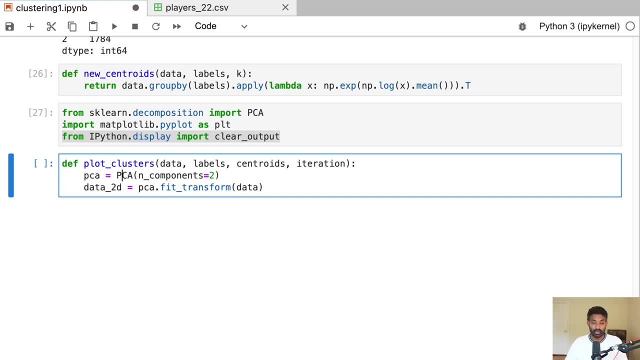 So we're initializing a PCA model and we're saying we want to have two columns returned by our PCA. So we're going to pass in data with several columns and we want that turned into data with only two columns And then the fit transform actually runs the model on our data. 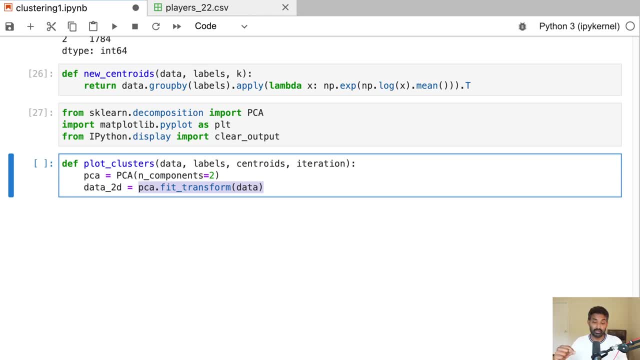 It first fits it to the data and then it transforms our data into two dimensional data. And we'll do the same with our centroids. We'll say: centroids 2d equals PCA dot, transform centroids dot t. And the dot t is because this PCA model expects our data to be in the form where: 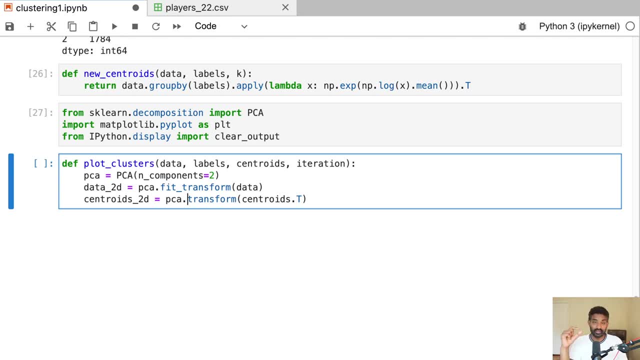 the columns are the features and the rows are the data points. So we're just switching our format There. then what we're going to call is clear output. So if we have a graph displayed, this will clear it out so we can display the new graph over it. 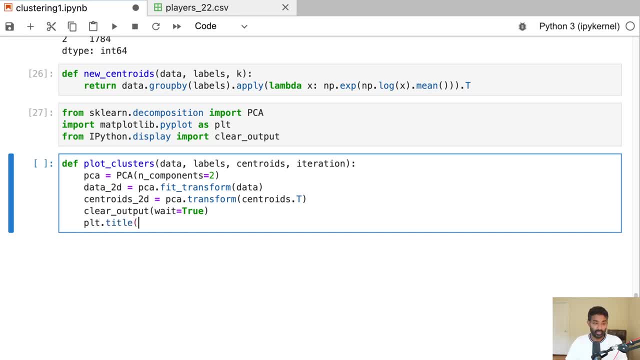 And then what we'll say is PLT dot title. So this title is just going to represent the iteration that we're currently on. Then we will plot each data point into our graph and color it according to which cluster The data point is part of. so data 2d- zero. 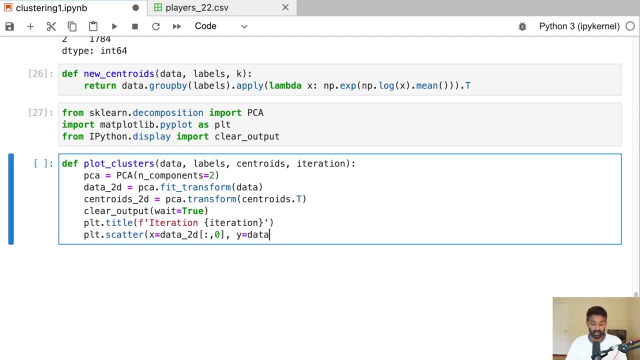 So that's going to be the X axis, And then the Y axis is going to be the second component that got returned by our PCA, And then what we're going to say is: color is the labels. So we'll color each point according to its cluster label. 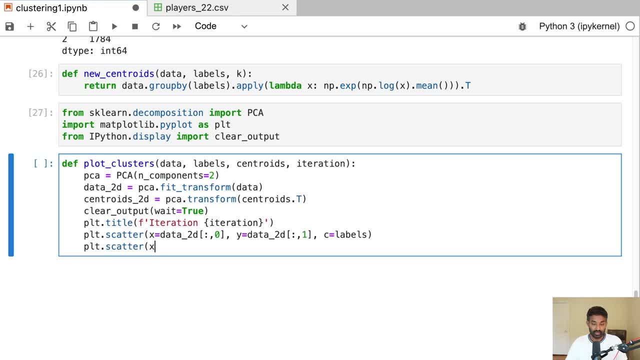 And then we will plot over top of that the centroids. So X is going to be centroids 2d Comma zero, And then Y is going to equal the second component, And then we'll call PLT, dot, show and that will show the plot. 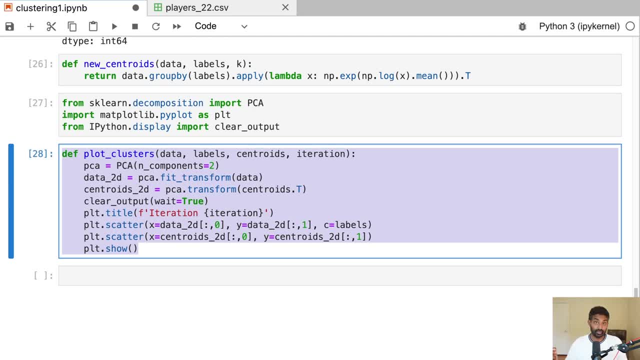 So it is not necessary to write this, but it's nice to be able to visualize the centroids and cluster shifting as the algorithm iterates. So this is first transforming our data Into 2d data, then it's plotting our clusters and coloring them and then plotting our 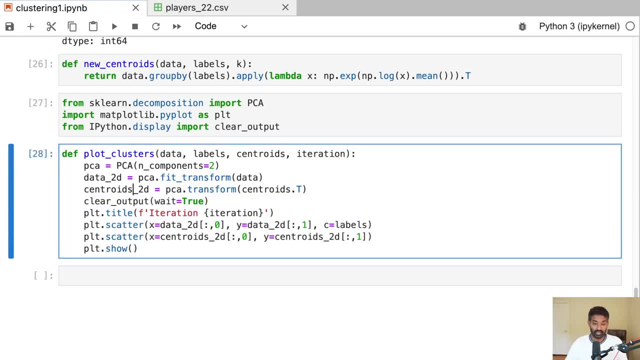 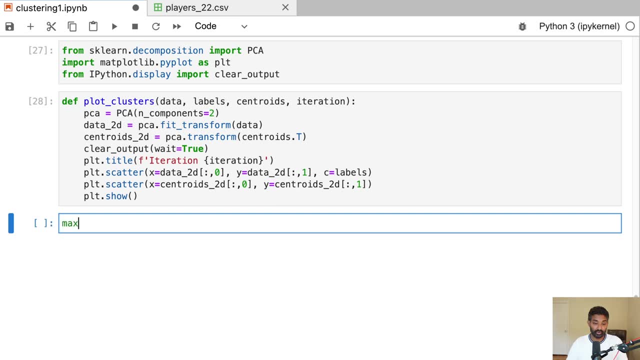 centroids, and then it's going to show the plot. So we'll call this at each iteration of our algorithm. And now we can actually go ahead and write the body of the K-means clustering algorithm. So we'll say: max iterations equals hundred, centroid count equals three. 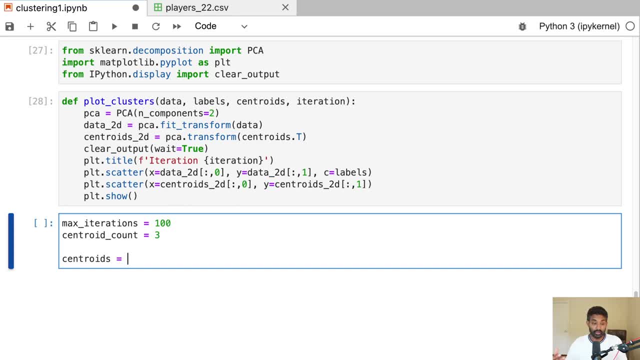 And then we'll go ahead and write our logic. So the first thing We're going to do is initialize our random centroids. Actually, instead of centroid count, I'll call this K, just to make it clear. So this is our number of clusters, and then this is our total number of times. 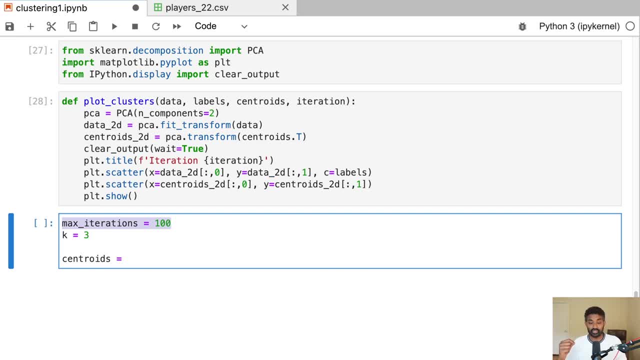 The algorithm will iterate unless the cluster stopped changing first- And I'll talk a little bit about that in a second- but the but. we will go ahead for now and initialize our random centroids, and that's just data and K, And then we will initialize our old centroids. 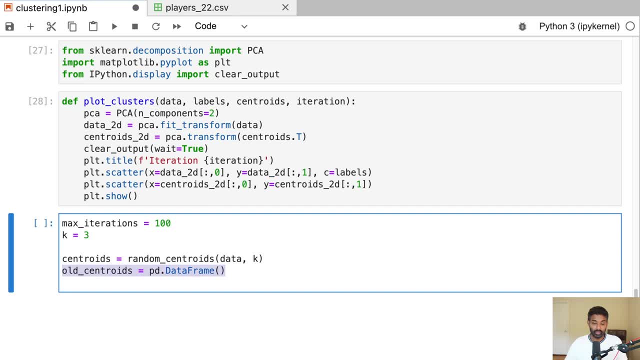 So we will stop the algorithm when our old centroids are equal to our current centroids, like that indicates that the centroids have stopped shifting. And then we'll specify that we're starting on iteration one. So we're going to say while iteration is less than max iterations. 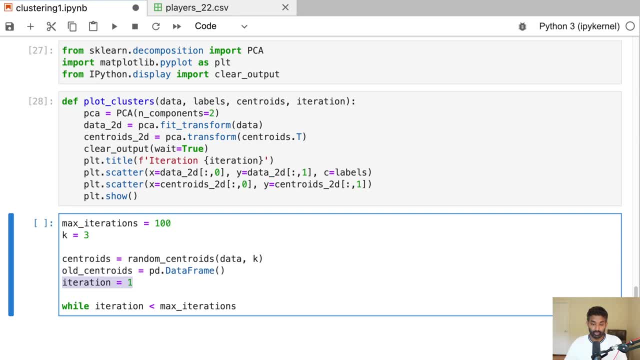 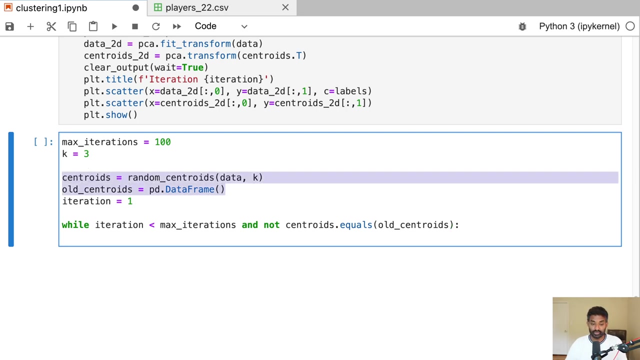 So, basically, if we, if our iteration counter hits a hundred, we want to stop our loop and and Not continue iterating our, our centroid values anymore and not centroids. dot equals old centroids. So what this is saying is stop the loop If we've hit our maximum number of iterations or our centroids are equal to our old. 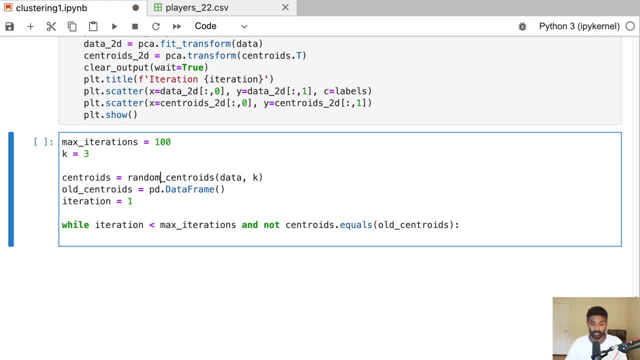 centroids, which means the centroids haven't changed in this update iteration. So we'll say: old centroids equals centroids. Then We'll Call our get labels function data centroids. So we we did this before, so we initialized our random centroids here. 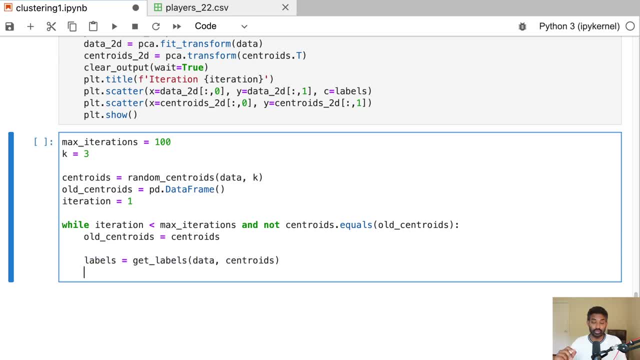 Then we're going to get the labels that correspond to each player, So we're going to figure out which cluster each player goes into. Then we're going to update our centroid values based on the geometric mean of all the players assigned to that cluster. 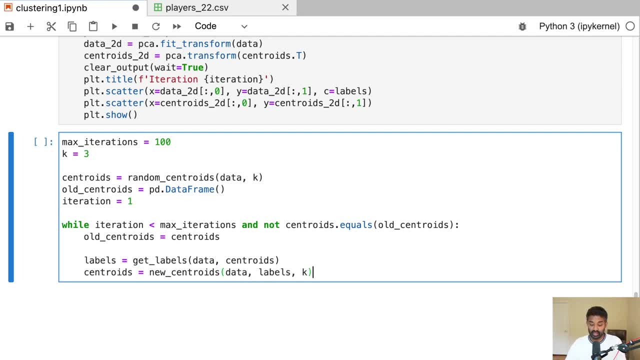 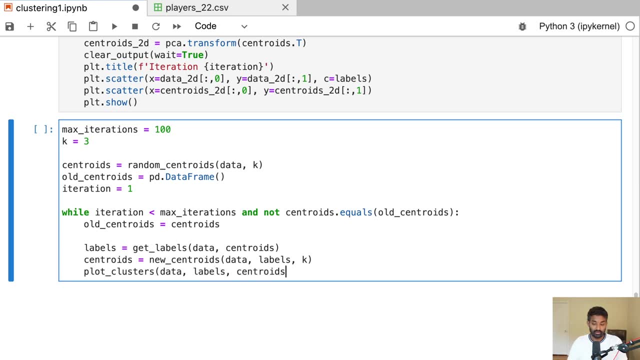 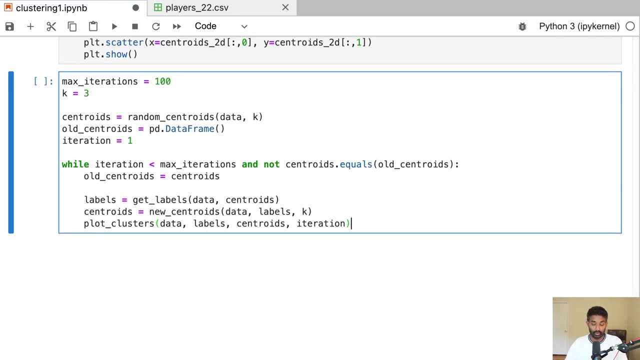 So in here, we'll pass in data labels, We'll pass in K, and then what we're going to do is plot our clusters. Okay, So a lot of this is just wiring together what we've already done, So this loop is basically just continuing. 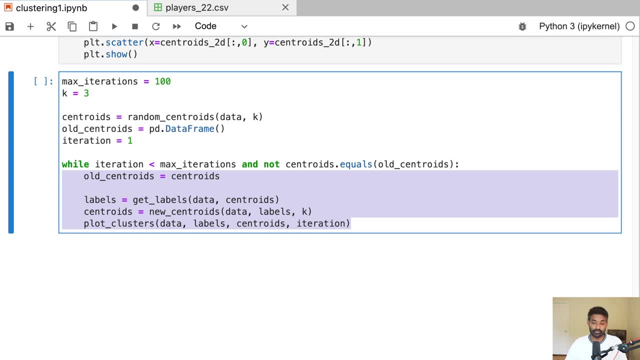 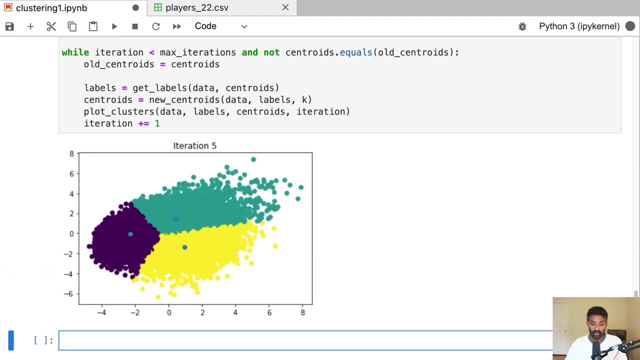 It'll keep running and it'll keep doing the steps that we already saw until it hits the stopping criteria, which are here, and then we're just going to increment our iteration counter. So let's go ahead and run this and we can see our clusters and we can see how. 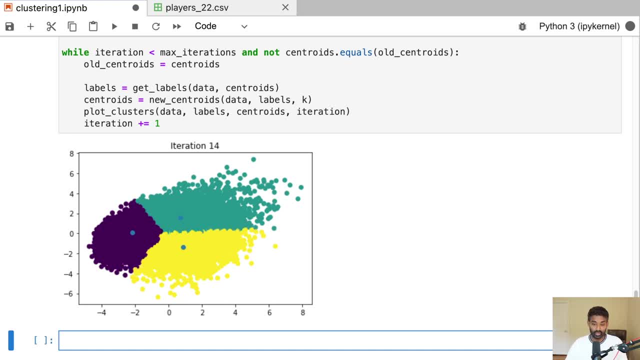 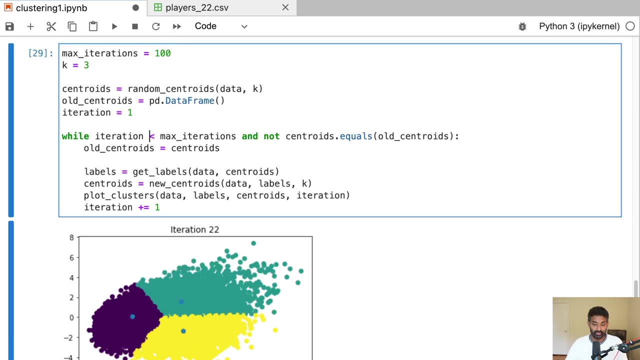 they change from iteration to iteration. So early on we saw that the clusters changed a lot. Now we can see that they're stabilizing. and then, around iteration 22,, the algorithm, the clusters actually stopped changing, So the algorithm stopped. I'll run this again just so you can get a closer look at what's happening. 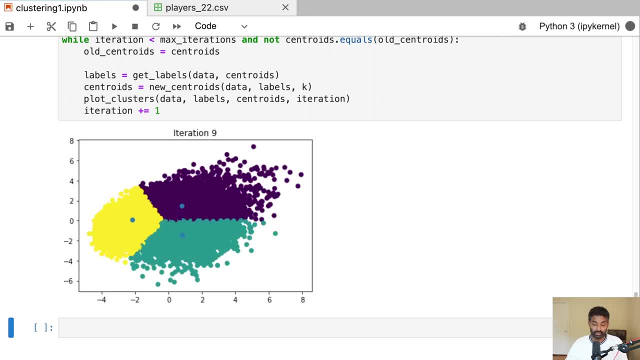 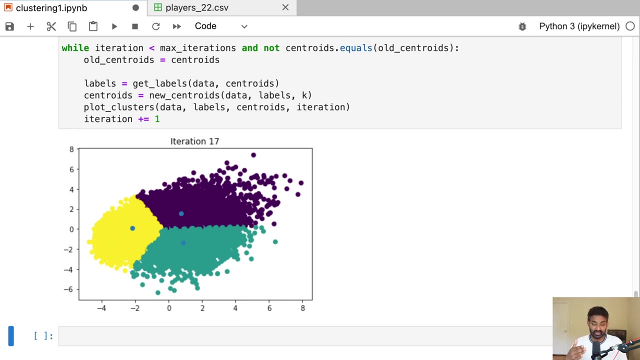 You can see, early on the cluster boundaries are shifting a lot. The centroids are shifting. later on It starts to stabilize and eventually it just stops changing The reason why the algorithm doesn't always result in the same output And sometimes it stops on iteration 17.. 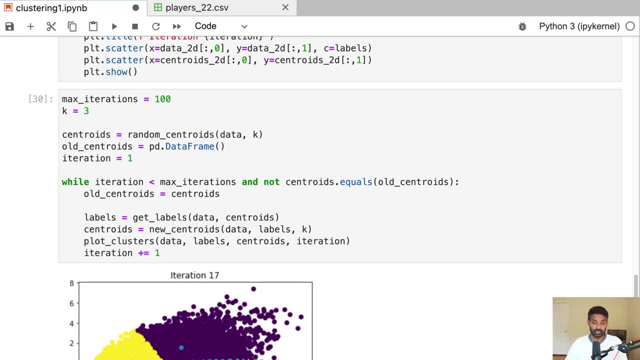 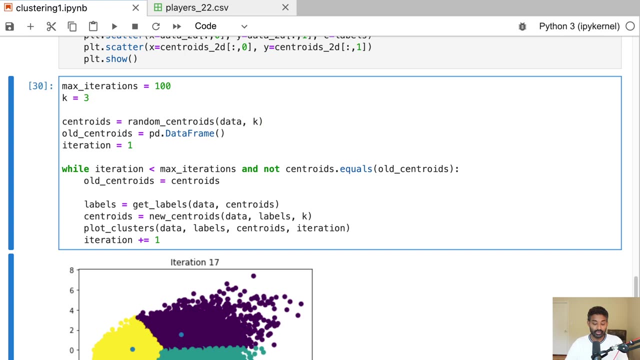 Sometimes it stops on iteration 22 is because the clusters are randomly initialized. so, depending on how the clusters start out, the algorithm could take longer or it could run in less time. Okay, And it really just depends on this random initialization. I can also increase the cluster count and we can see how that changes our graph and 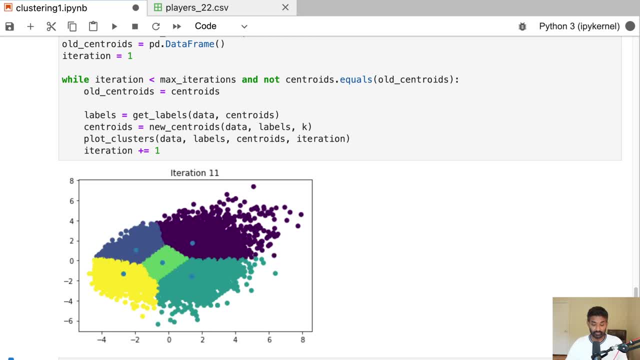 how it changes the cluster convergence. So kind of cool. We ended up with one cluster in the center and the rest around the outside And generally the more clusters you have, the longer the algorithm will take to converge. So you can see it's going through more iterations here to try to stabilize. 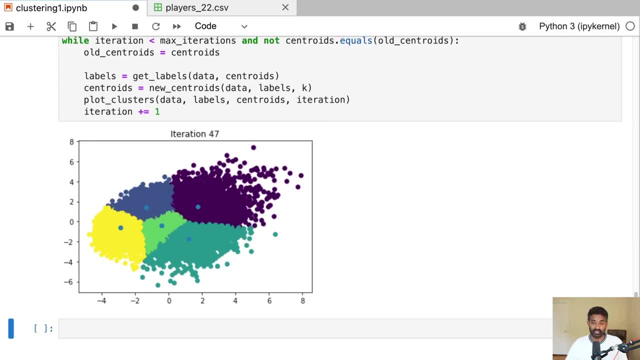 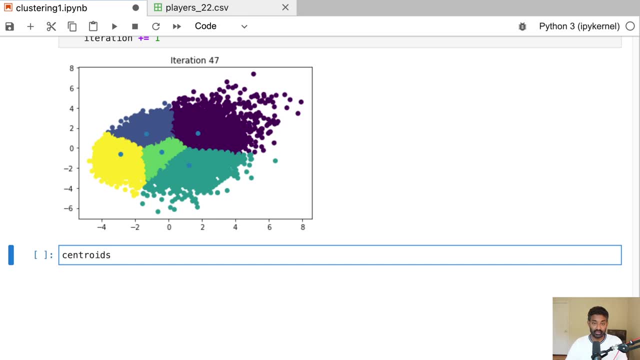 Okay, And then at iteration 47,, that's when it stopped changing and the algorithm ended. Once the algorithm ends, we can take a look at the centroids and see what they represent. So this is the fun part is interpreting the output of this. 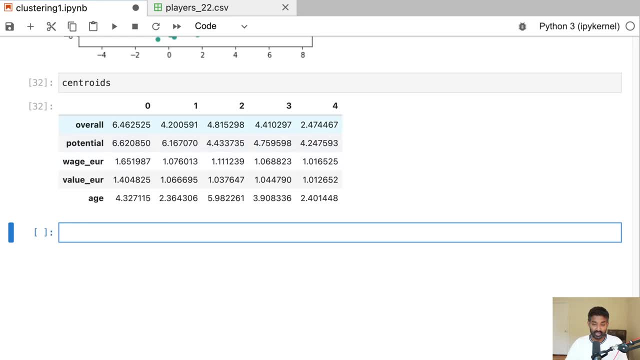 So you can see from the clusters each cluster has slightly different values for each of these key columns. So you can see cluster zero here represents star players. So these are players who the age is kind of in the middle of the distribution, So they're in their prime. 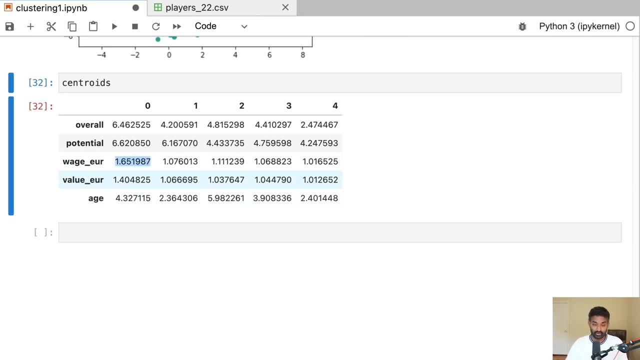 Their wage is pretty high relative to the the other, the wages in the other clusters, and their overall and potential scores are actually high as well. So we can confirm this hypothesis by looking at players label labels equals equals zero And we can see which players this is actually referring to. 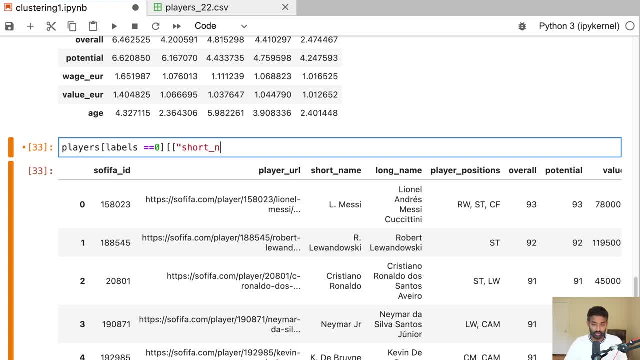 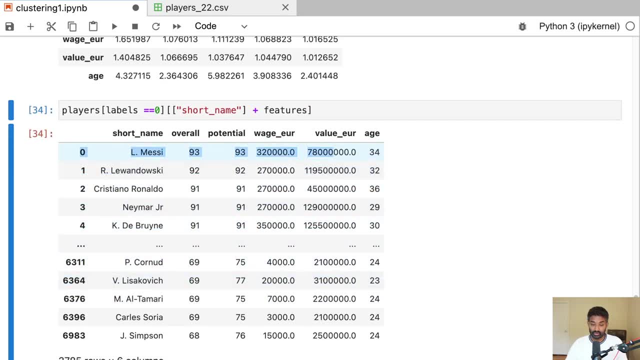 And let me actually look at Fewer columns So we can look at short name plus features. Okay, So we can see these are star players, right? So this is players like Lionel Messi, Cristiano Rinaldo, Neymar, et cetera. 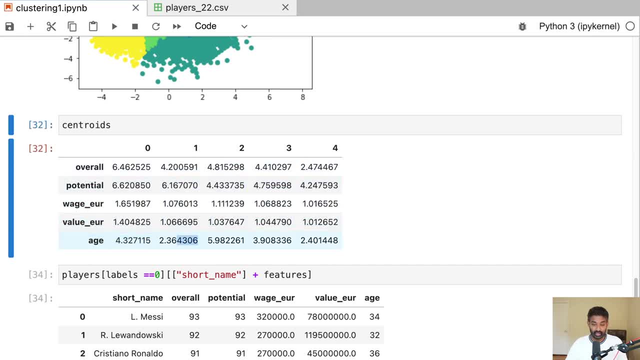 Cluster one looks like younger players. You can see that the age is. their age is lower, Their salaries are also lower and their overall rating is is lower than than average, but they have high potential. So Let's take a look at this. 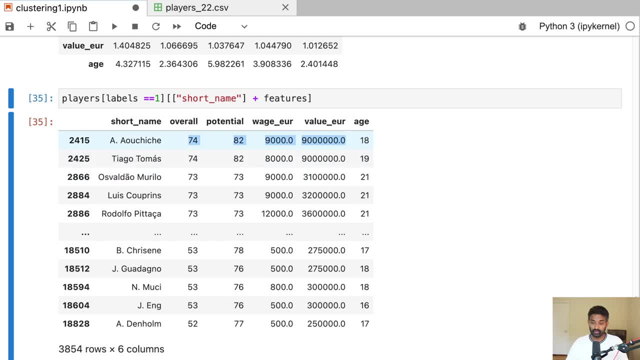 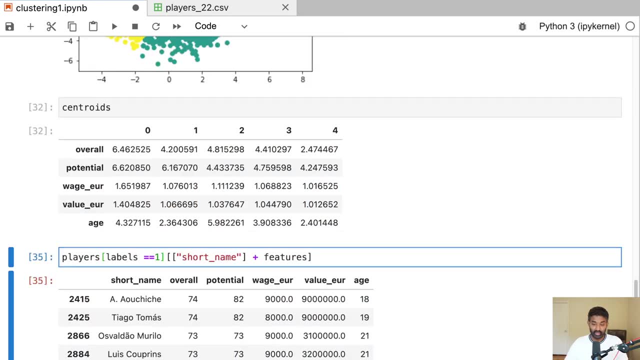 And we can see that these are all players who are younger, Like their age is pretty low but they have high potential. And then we can also look at cluster two. This appears to be older players, So their, their age is kind of greater than the other clusters and their overall and potential. 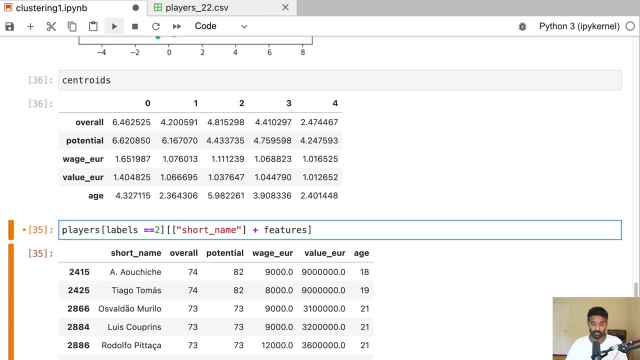 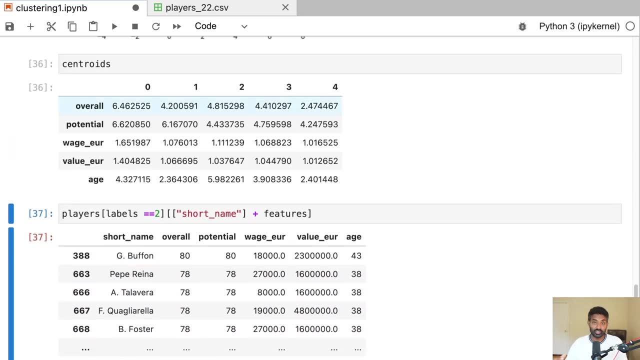 are about the same, So we can take a look at this as well. Yep, So we can see These are players who have hit their potential and are are older, And so on. So once you develop your, your, once you finish running your algorithm and you get the values, 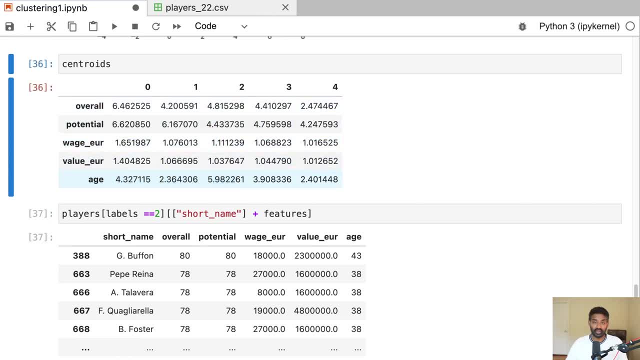 for each cluster, you can actually go ahead and start to interpret it, And that's the really cool part about K means is it can find patterns in your data that maybe you didn't know were there, And if you follow football, you you may know of some of these patterns, but one it can help you. 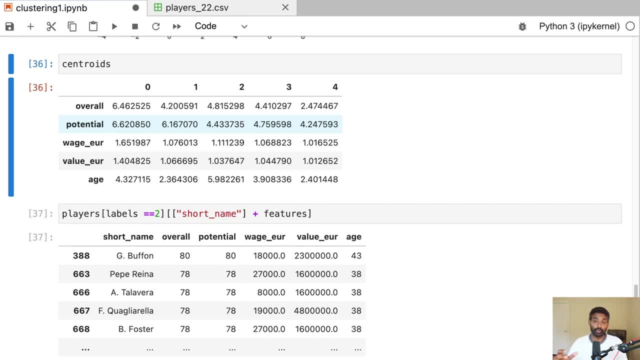 automatically categorize players into each group, So you can then process them differently. If you're building a system to, for example, rate players or do something along those lines. And then two, it can help you find patterns that you can use in your business or to 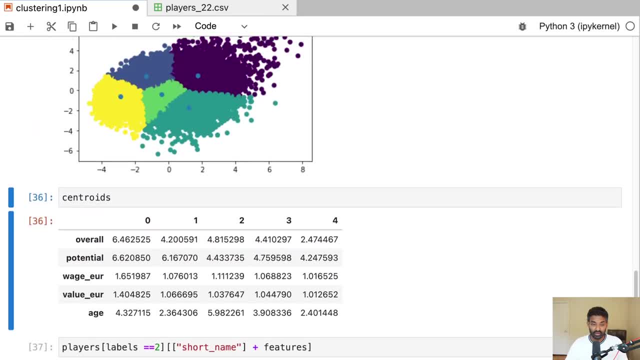 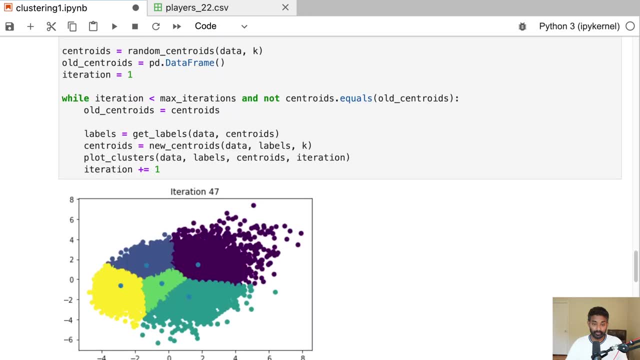 to draw interesting insights. So those are the centroids. The next thing we can do is just compare what we did to the scikit-learn algorithm. So I'm going to go ahead and reduce the cluster count to three. just makes it a little bit easier to. 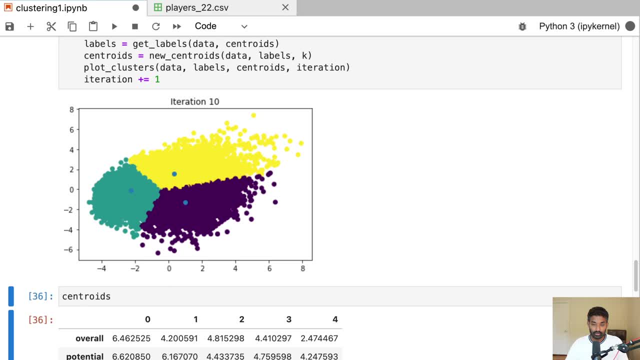 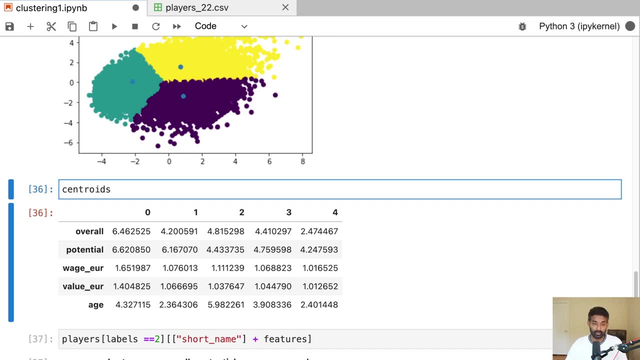 compare So we can see the algorithm is running, and then I'll, once this finishes running, I'll take a look at how the actual cluster assignments shook out, or how the actual centroid shook out, Okay, And then we can see our centroids here. 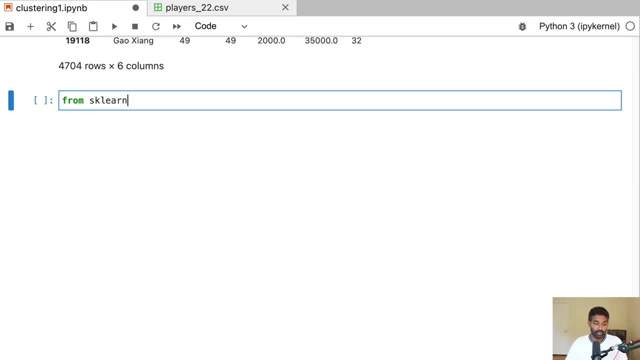 And then what we'll do is we'll just compare this to the implementation that's in scikit-learn, just to see how we did So. to initialize this, we do k-means three, So three specifies the number of clusters we want. 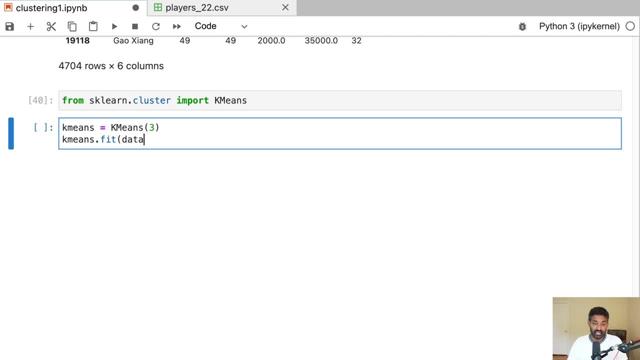 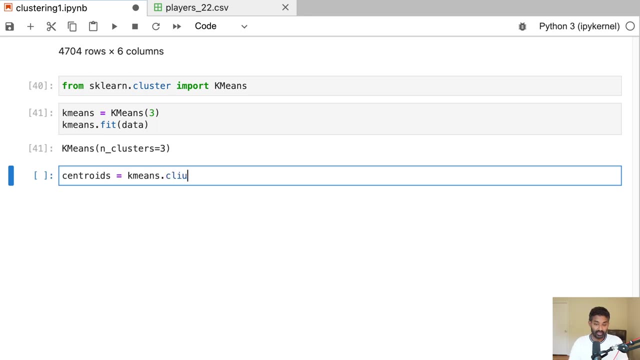 And then what we call is k-meansfit data. And then what we to get the centroids? we say centroids equals k-means dot cluster centers. And then we can create a short small data frame here to actually look at the centroids. 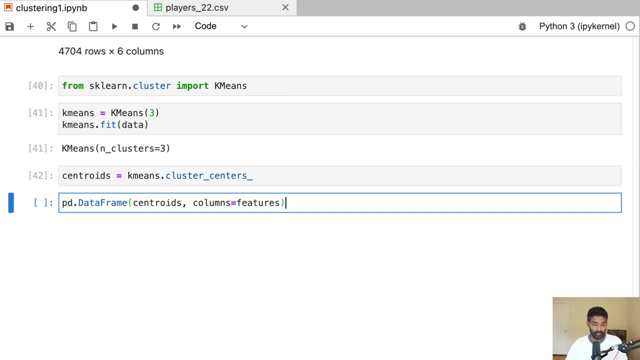 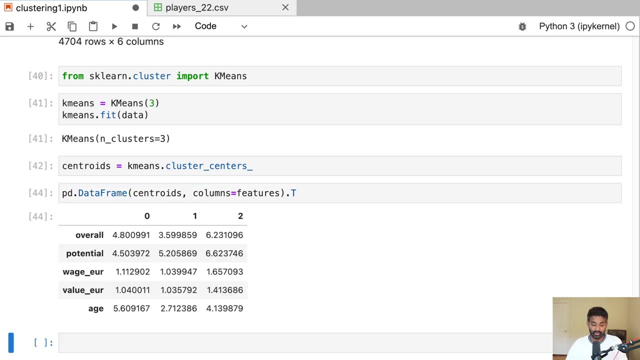 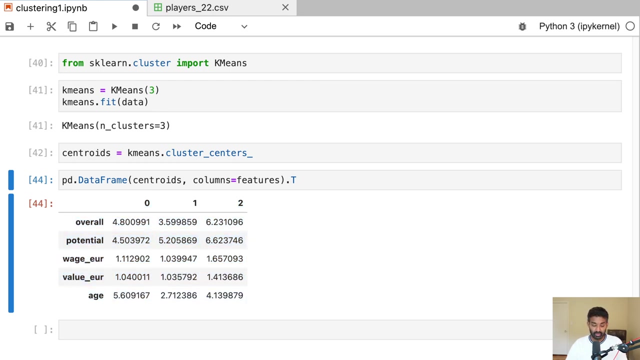 and specify the columns. So the columns are going to be the features, And then we'll just turn this so it looks like our other centroids. So each column is the centroid and each row is the feature. And then if we compare this to what we got before, which I'll drag down here, 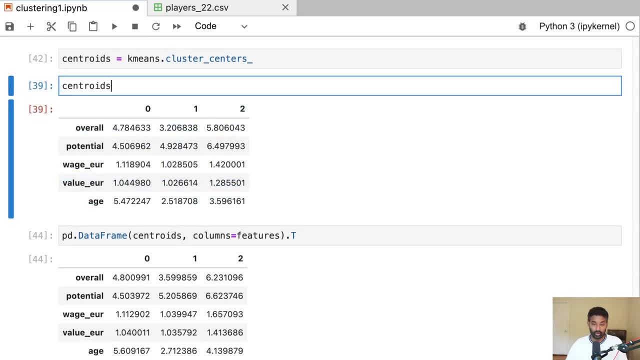 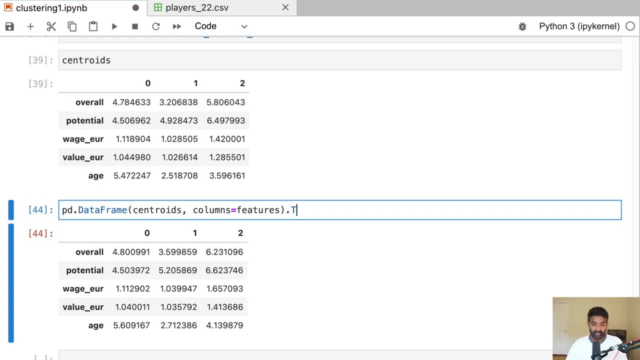 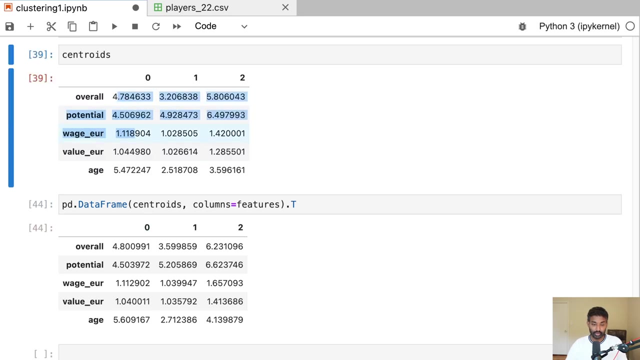 So these were our previous centroids that we got with our algorithm And these are the centroids that we ended up getting with scikit-learn, So, Okay, So we can see a lot of the same patterns, right, So there is cluster zero. in both is a group of players who've kind of hit their peak rating. 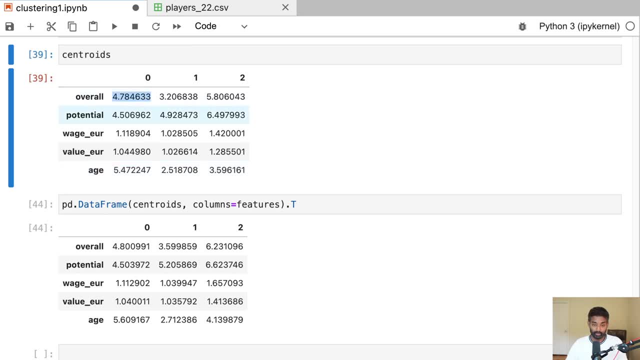 They tend to be older and they they're overall and their potential are about the same. Cluster one is younger players who are still rising. They still have a lot of potential, And then cluster two is kind of these star players who make a good amount of money and are close to. 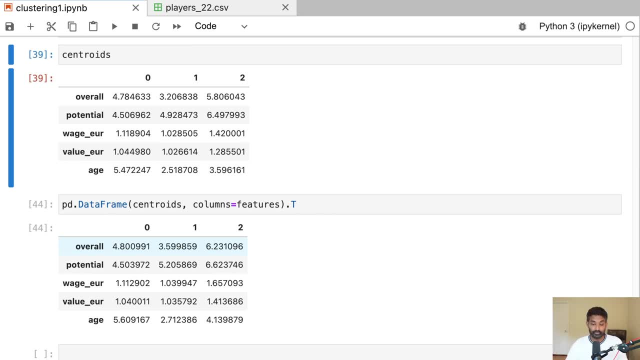 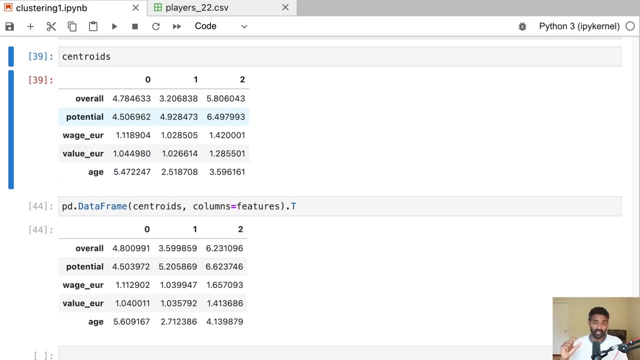 their, their, their potential rating. They're in their prime, still All right. So the values aren't the exact same, because the underlying algorithms are implemented slightly differently and the randomization that I mentioned before. But they're close enough that we have some confidence that our implementation is working. 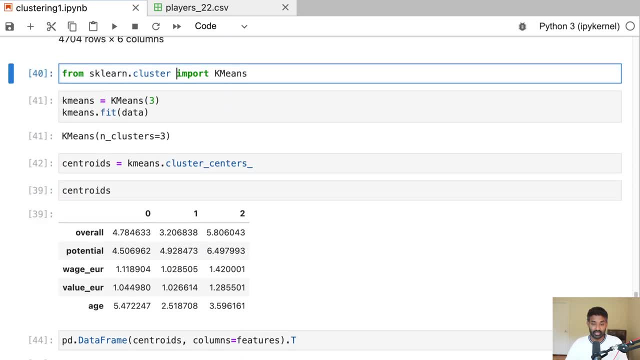 Okay, And seeing how quick it was to run this in scikit-learn, why would you want to build your own K-means cluster? Right? so there are a few reasons. so one is learning, so implementing your own k-means clustering algorithm. 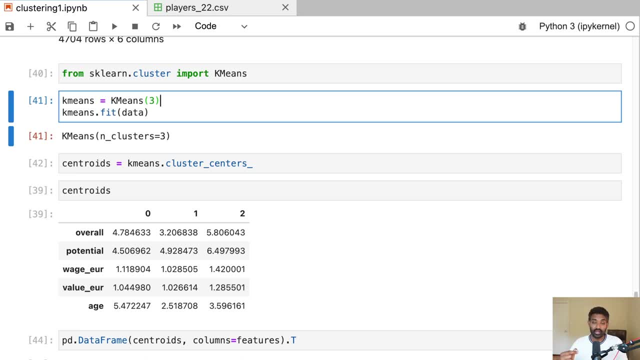 is the best way to learn how it works under the hood and really know which situations you can apply it to and which ones you can't. another is that it gives you more power and flexibility. so if you wanted to modify this k-means algorithm to work in a low memory situation, work on multiple 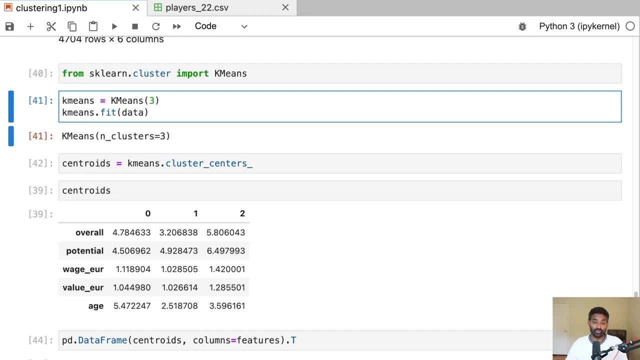 machines, etc. you can do that with your own algorithm more easily. it also looks good in a portfolio if you implement an algorithm on your own. it can also look good during interviews if you're able to talk through how an algorithm works. in a lot of data science and machine learning.